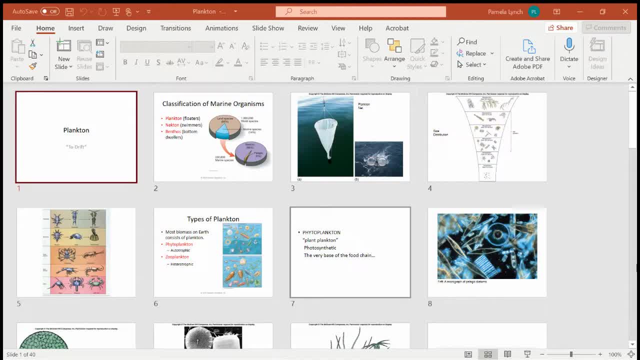 your lawn, like the trees and the flowers and plants outside, they form the base of the food chain. Without plankton in the water, you would have nothing else. So I like to start the discussion of marine biology by introducing a specific type of marine organism, namely plankton, And that's. 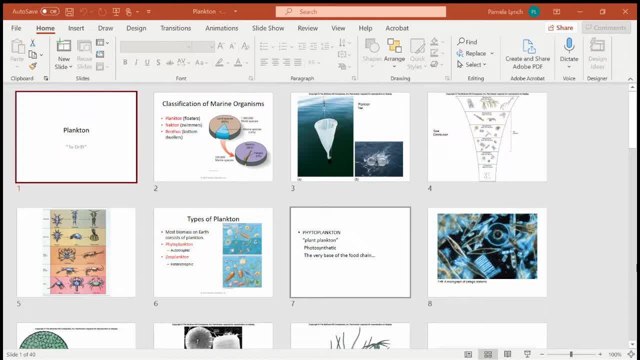 also why you do a specific lab about plankton During the plankton lab, lab number 10, your focus is on primary productivity. Now you may not have been able to put two and two together about what plankton and primary productivity have to do with each other, But if you remember back to your basic, 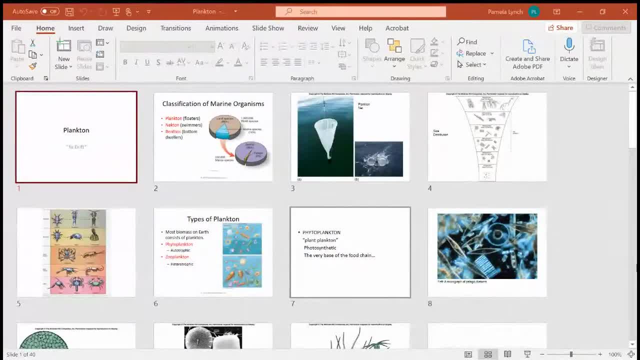 trophic structures, your basic food webs. in middle school even right, You know what a producer and a consumer is. Producer is something that produces its own sugar- It doesn't need to eat anything to get energy. And a consumer is us something that has to eat something else. I can't go outside and 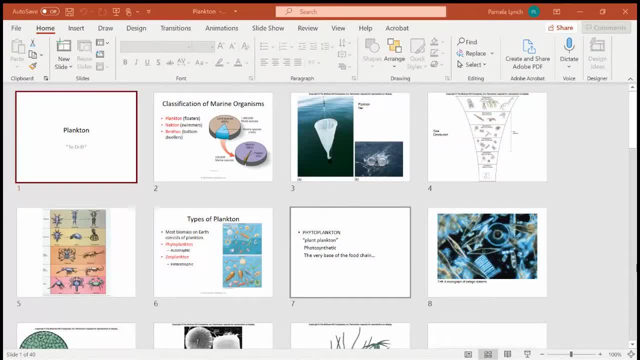 stand under the sun and have lunch right. So a producer is something that literally produces food In lab 10, you're measuring primary productivity. Productivity is production producer. So it's basically letting you know about the plankton level, particularly phytoplankton, those which are photosynthetic, those which are 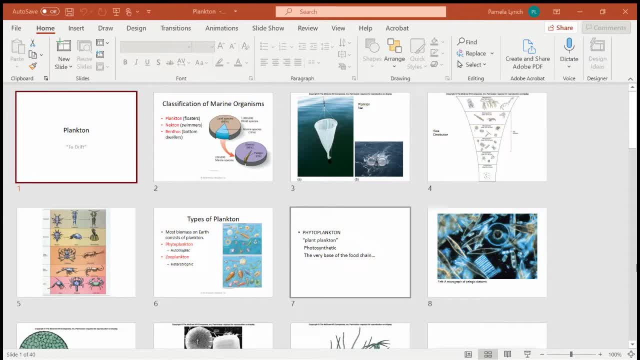 producers how much of that is in the ocean. And they change based on the seasons, and they change based on temperature, based on location and based on temperature, based on temperature, based on nutrient input. Again, all stuff that is related to lab 10.. So not only are we introducing a marine 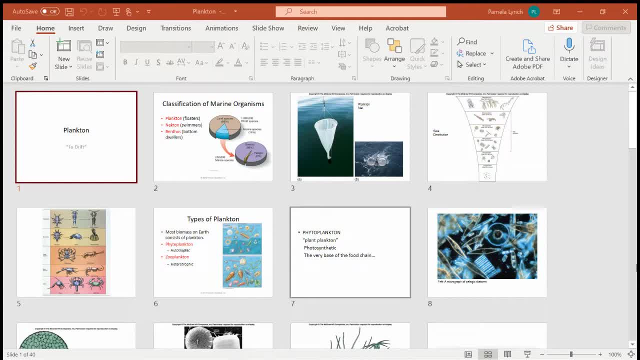 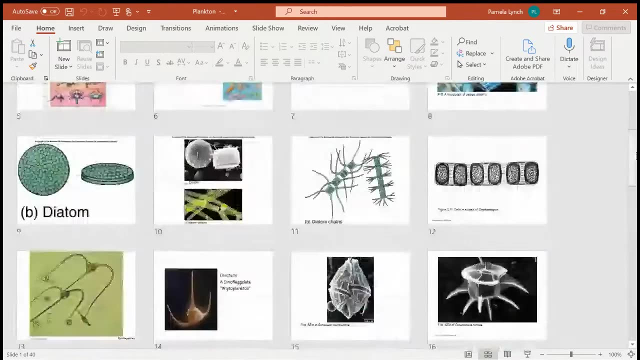 biology topic and a very specific subset of marine organisms. we're tying this in with the lab 10 material. okay, So this lecture is pretty comprehensive. I'm just going to scroll and show you all of the different pictures. right, There's a lot of pictures here introducing to you to what 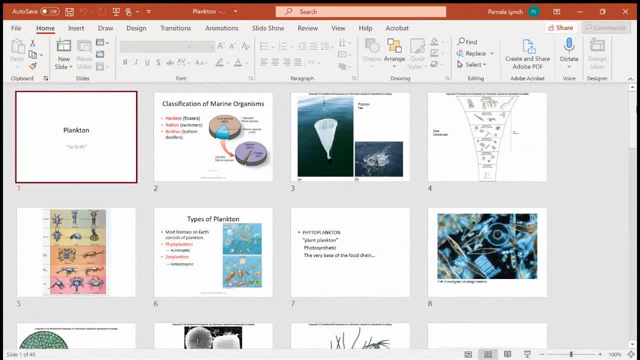 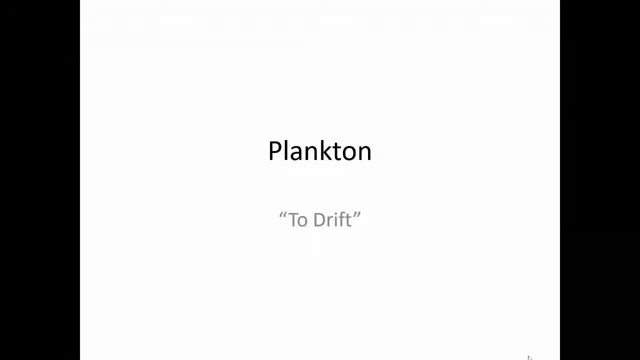 these concepts are. I'm just going to briefly highlight these concepts so that you can better understand the concept of a marine biology topic and its role. So, most importantly, when people say the word plankton, or when a biologist says the word plankton, we automatically think small right. 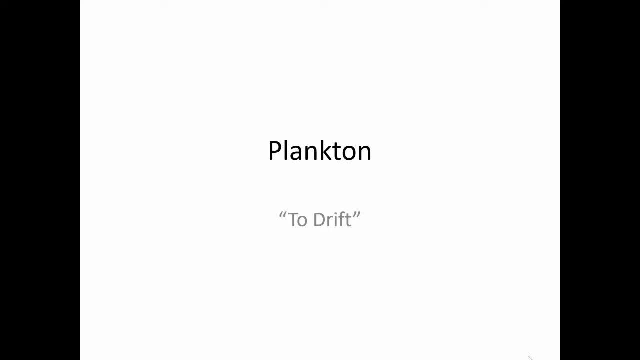 Because they're almost always the microscopic stuff in the water. But it really doesn't mean small And there are large, 100-foot-long plankton. So while there are a lot of small plankton, it doesn't mean small. The definition is not small. The definition actually means to float. 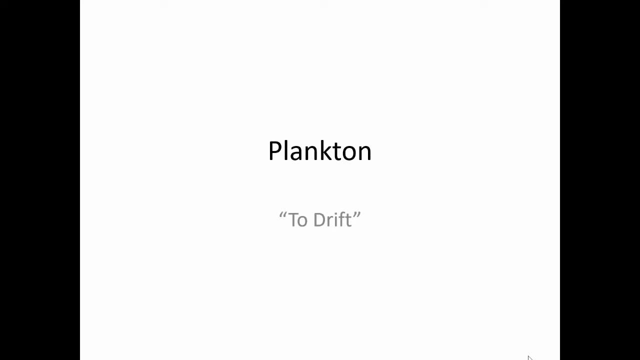 or drift. So it's a definition of a marine biology topic. And it's a definition of a marine biology topic. So it's a description of mobility, a description of movement. If I were to go outside and lay down, my description is laying If I sit up, sitting, If I walk, walking, If I skip or hop. 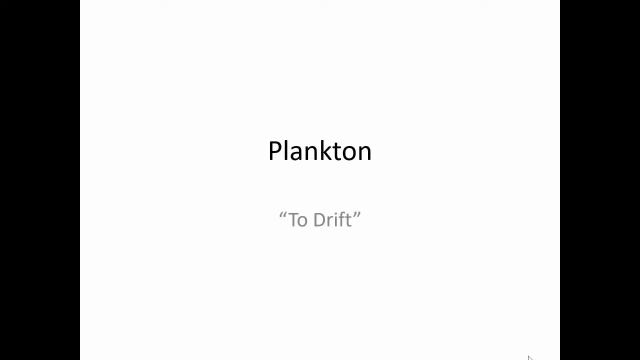 or jump or run. I'm describing what I'm doing, If I'm drifting. that is what plankton are doing. What it means is that if you have these organisms in the water and the waves or the tides or the ocean, energy is moving the water in a certain direction and you go to the ocean and you go to the. 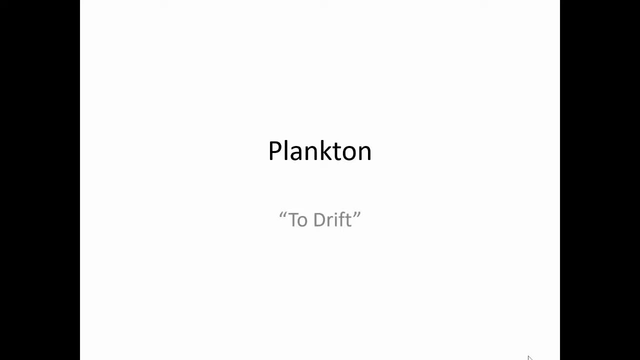 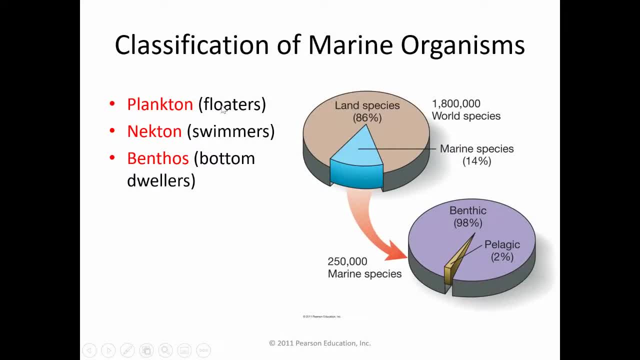 which the water pushes them, So we call them the floaters of the ocean. The, of course, opposite organisms are those that can swim. The term for those are nectid. So those are two marine biology terms that you're responsible for knowing, Okay. 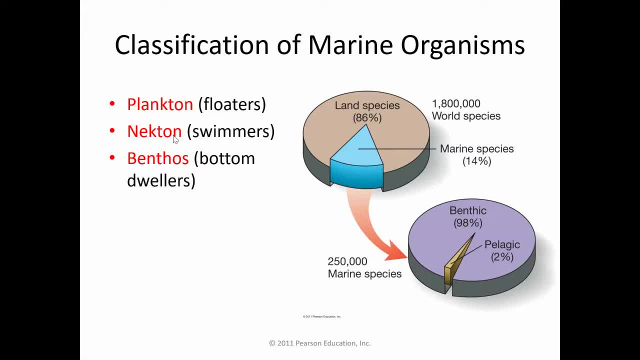 Plankton and nectid And, by the way, you in the ocean can be both. If you jump in the water right now and you do dead man's float and you float around, you're being plankton If you actively swim through the waves and you go in the opposite direction to which the waves are crashing and 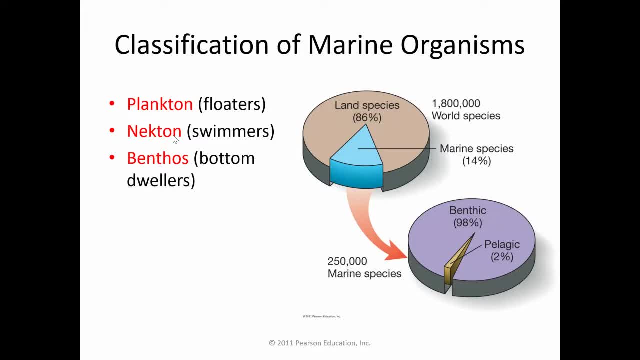 you're swimming, you're nectid. Now those are, if you're in the water- column right, Meaning in the actual water- you can either swim or float. The third type, and again the third marine biology term that you're going to need to know, is called benthic. 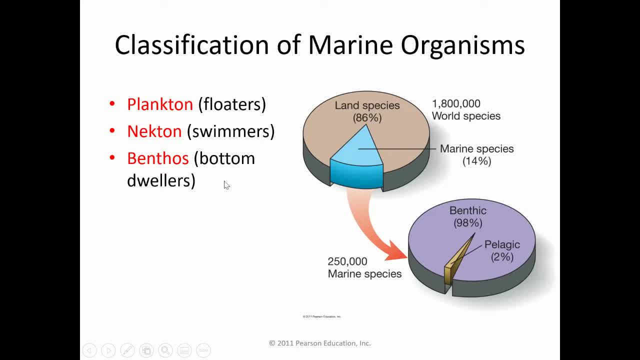 Benthic is plural. If you're not in the water physically, in the water column you might be standing, or attached to the bottom. You might be landing on the bottom to feed. You might be crawling out into the intertidal zone, right where the waves are splashing to feed rest nest. 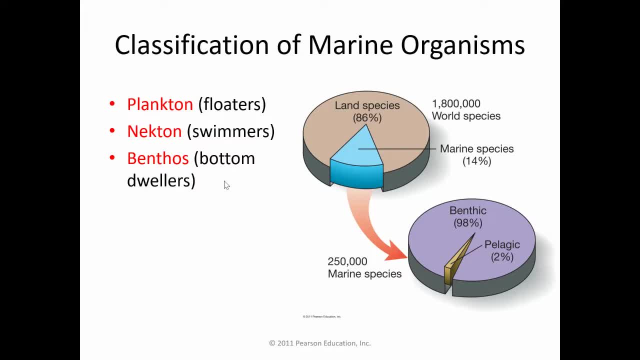 breed, mate, whatever, considered benthic. So those are three key terms And, of course, what I'm going to do in this lecture is introduce to you the concepts and the organisms that fit in these categories. Okay, we're going to start, of course, with the topic right now. 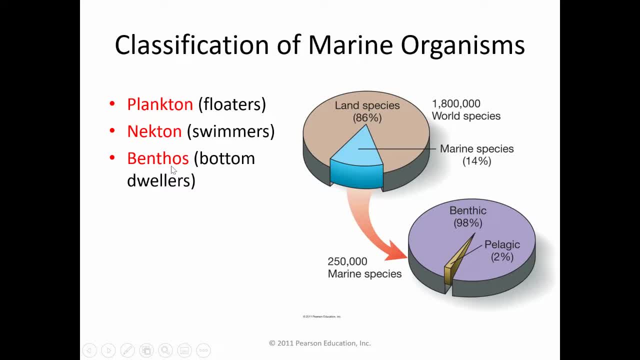 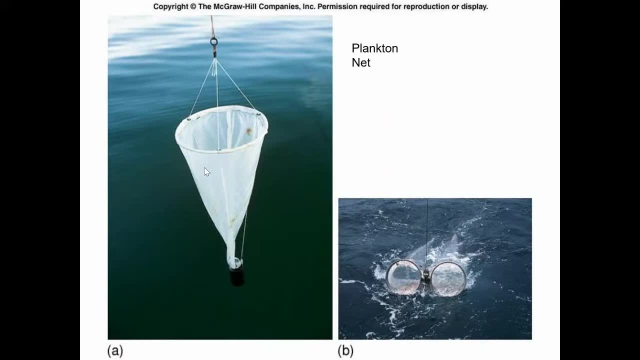 which is plankton. I just wanted to remind you that these two other terms are coming your way as well. So, specific to plankton, the way that we collect plankton are with these things called plankton nets. They're like really fine mesh pantyhose, really like the finest mesh pantyhose. 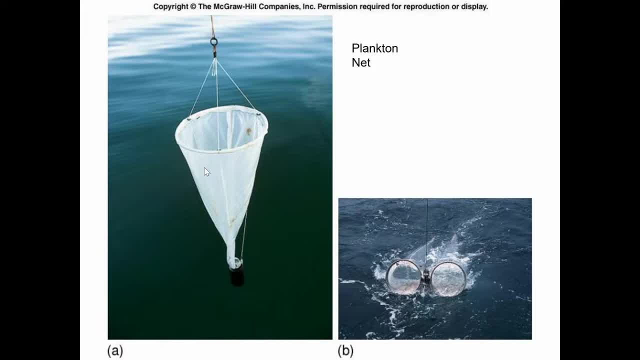 you can have. So it allows the water to go through. but the organisms are just a little bit bigger than the mesh of the net And they get collected in these little glass jars that you can see here and we can put them under microscopes and be able to see them. So you'll see, now that the size 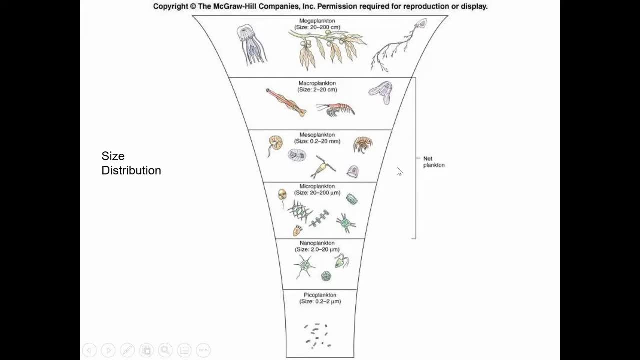 distribution is pretty vast. Most of them are microscopic, right, All of these. you would need a microscope to see. Some are macroscopic, like these: Okay, look, shrimp. you guys know what these are, right? Shrimp, jellyfish, salps, comb jellies, arrow worms- these you can see visibly. 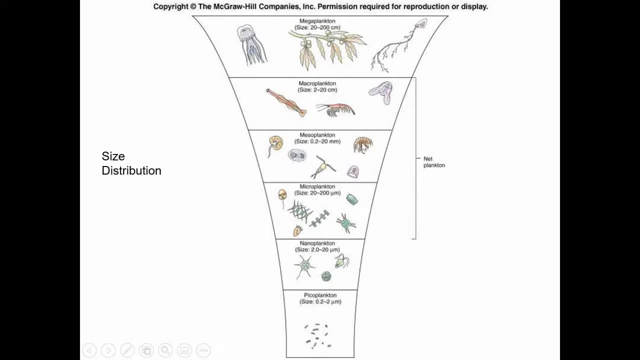 with the naked eye. Even some copepods you can see with the naked eye as well, or amphipods, But by and large, most of this stuff is not visible. So what we're going to do is we're going to do is we're going to use a microscope to see if there are any organisms that can fight the tide. 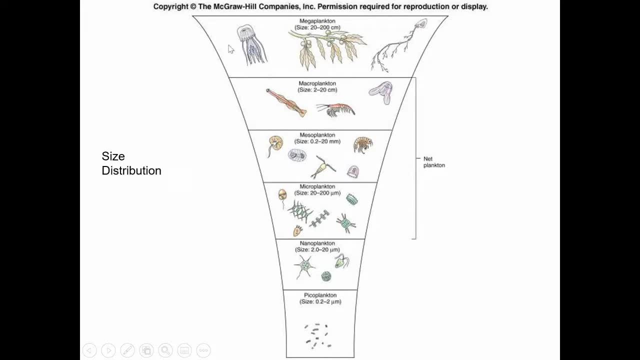 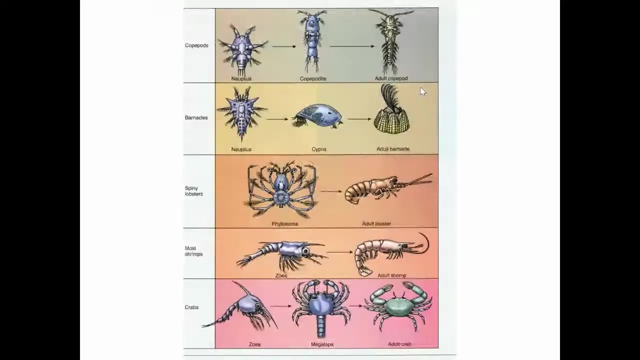 So just a quick reminder as we move through: while a lot of the plankton is microscopic, it doesn't mean small. Another thing that I want to point out to you guys is not only is plankton a definition for a mobility type- to float or drift, it also, more often. 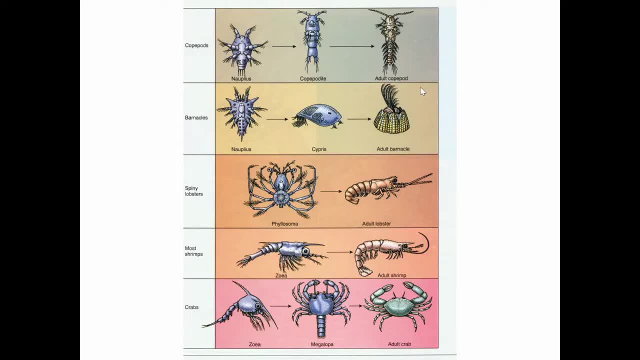 than not describes a life cycle stage of an organism. So most of you know what a barnacle is. You've seen them on the sides of a whale, or on the sides of a boat or a bulkhead. Everyone, I hope, knows what a lobster or a shrimp or a crab is. But, believe it or not, this is what 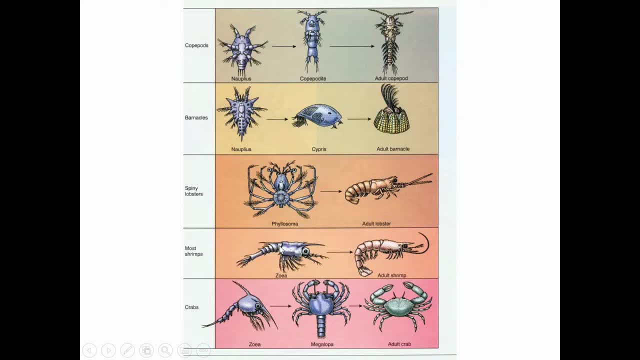 they look like in their juvenile stages. in their larval stages They look dramatically different. Those are their planktonic stages. We again are very similar. right When we're in your mom's belly, we look totally different. right As a fetus, we look different. 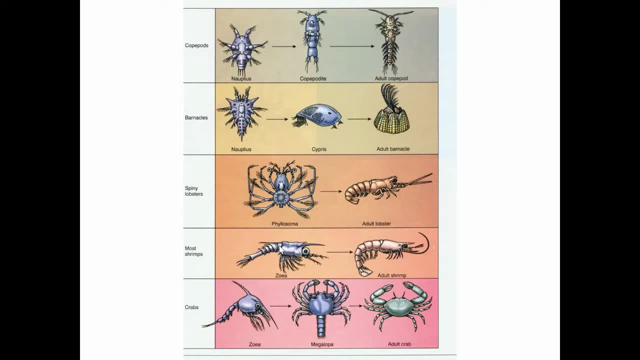 When we're born. think about, you know, when you come out on your first couple of weeks of birth, you look like an elf, right. You look kind of a little bit different than you look now. You have a different stage. Then you go through the infant stage, the toddler stage right, And 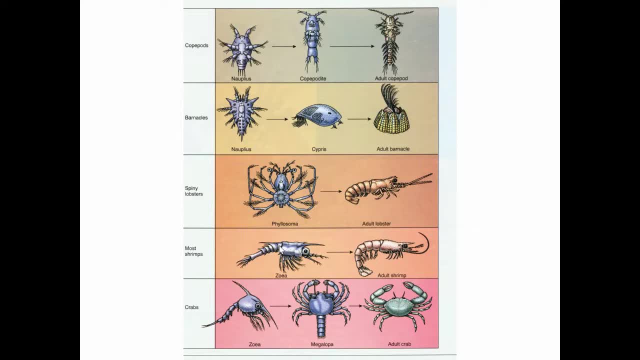 there's all these different stages and they describe essentially our age but also our ability. We eat different things, We can move different, We have dependencies on people differently, based on those stages. So you know, we're in your mom's belly. We look totally different. 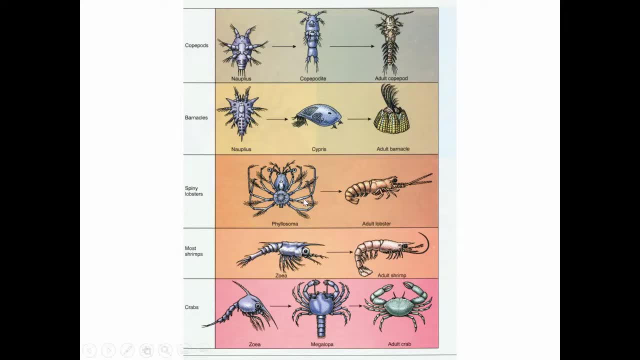 Plankton are no different. So a juvenile lobster right here. this is floating and drifting and cannot move against the current. An adult lobster is benthic. It settles on the bottom floor right. Barnacles become permanently attached. Here's their adult stage as a benthos. 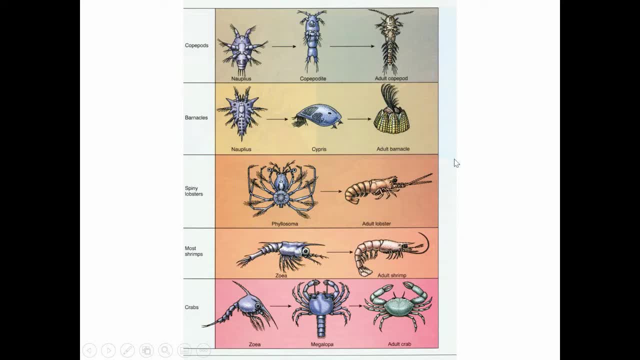 They start off planktonic, So plankton again can represent not only floating and drifting a description of what they're doing, but a life cycle stage. And they're critically important in all of those different stages, not because they're growing. that's important as well. 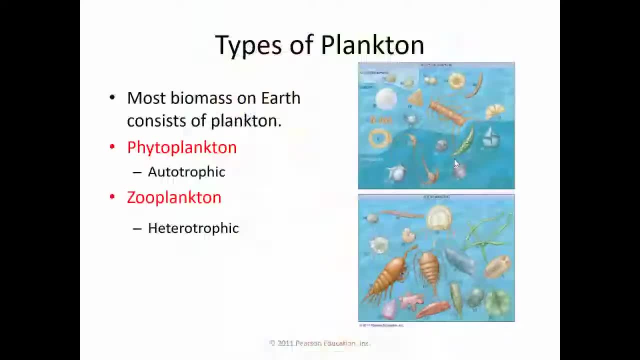 but because they're the food source for a lot of stuff when they're in those planktonic stages. Now here's another two words that you're responsible for knowing. okay, We've already seen the word plankton, right, So plankton is at the end here of both of these, But the leading 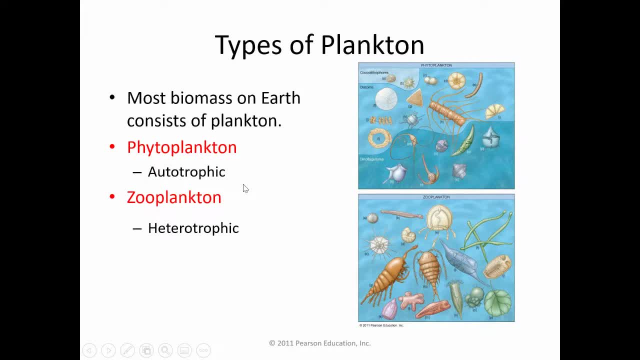 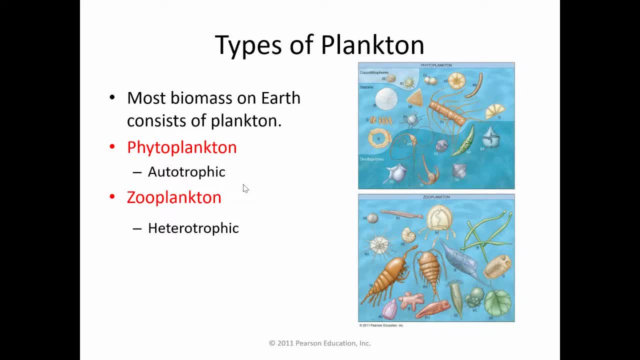 and autotroph. That means it's a producer. That means with the sun, it can produce its own energy. That is the primary production that you're studying in Lab 10.. If you're not an autotroph or a producer, you're a heterotroph. Heterotroph means consumer. That means you have to eat. 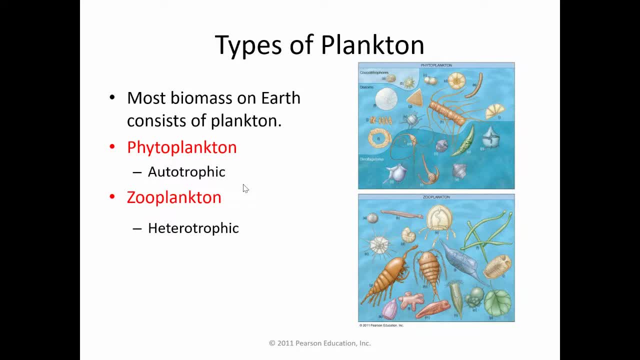 something else. So zooplankton animals in a zoo, right, Those are the animals. Animals are always consumers or heterotrophic. Remember these fancy words: Trophic means feeding, So a food web is really a trophic web. 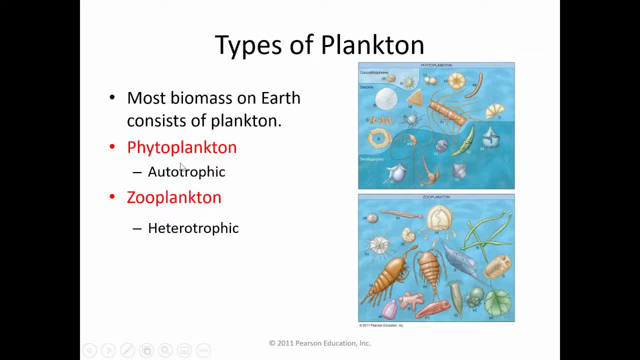 okay, So that's the feeding portion. Auto means automatic, So you automatically make your own food. Hetero means other right. If you're a heterosexual, you like the other sex. So heterotrophic means other feeder. That means you have to eat something else to be fed. 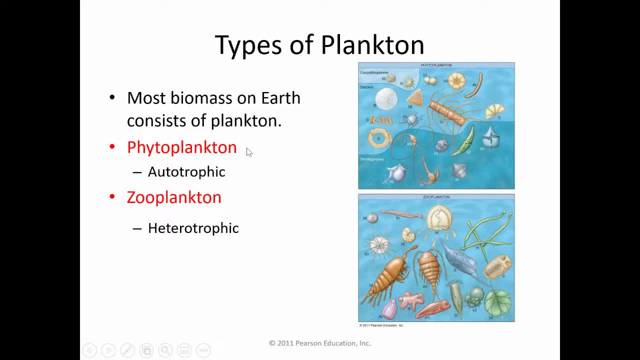 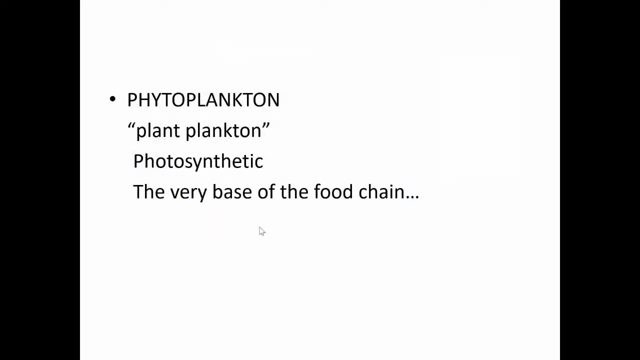 as opposed to automatically being fed yourself. So two types of plankton: phytoplankton and zooplankton. Phytoplankton are the ones responsible for primary productivity. I'm going to show you guys some super cool pictures of phytoplankton. first, The classic definition for phytoplankton: 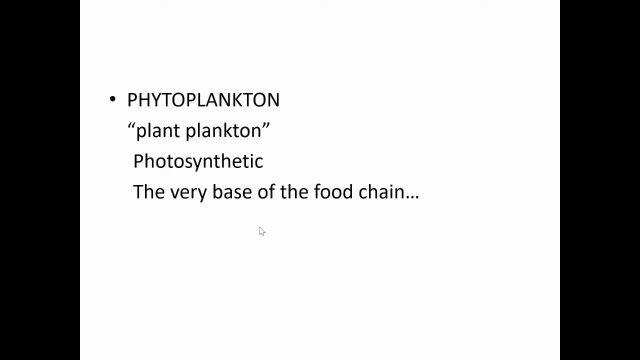 again is to float and drift And we usually call them plant plankton. That's a little bit of a misnomer And as a marine biologist I don't actually like that, because they're not plants, They're not in kingdom plantae from a classification perspective, but simply because 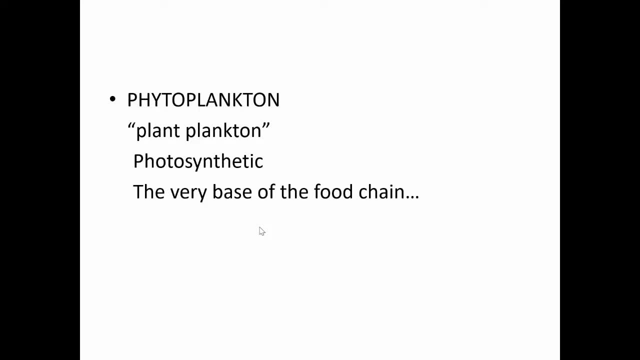 they photosynthesize. people like to call them plant plankton. It really makes more sense to call them algae, But because they're photosynthetic and they form the base of the food chain, they get that misnomer as a name. As long as you guys know that they're autotrophic, meaning that they're 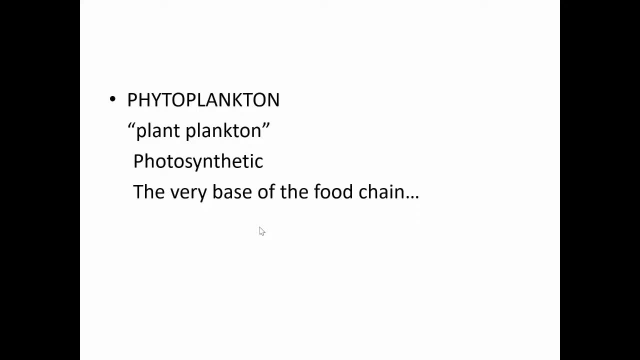 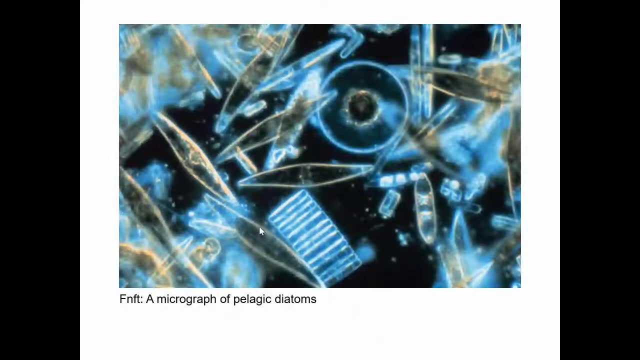 producers based on photosynthesis and that they're the primary producers of the base of the food chain. you should be good. Here's some cool pictures. So there's four or five different classic examples, but the two main ones are called diatoms and dinoflagellates Di two. 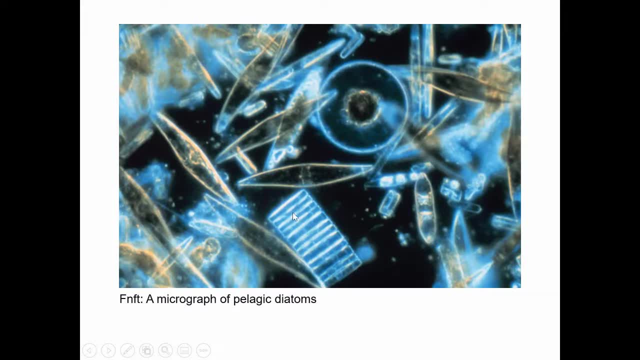 tombs, like two disks Stacked. Sometimes they come in groupings as well, But more often than not they just look like stacked pancakes, stacked disks. You can see that they're clear. Clear, obviously, is important. They're made of silica or a type of glass. If they weren't clear, how would the sun penetrate? 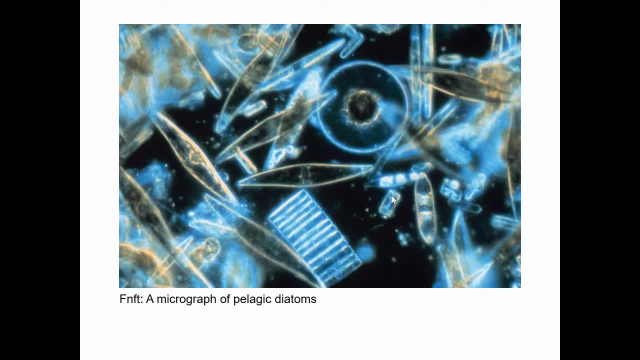 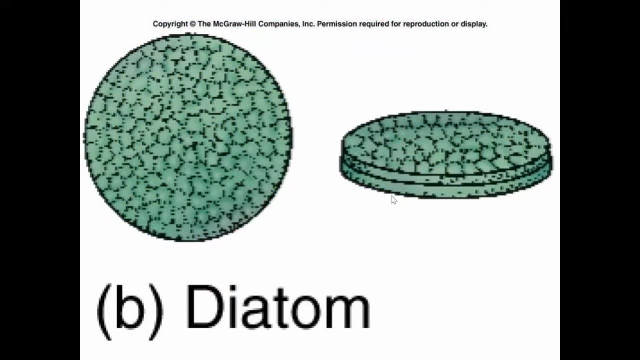 into their body so that they can make chlorophyll right, So that they can actually produce their own sugars. So all of the phytoplankton you typically see are clear. Here's a schematic. You almost always see them green representing the chlorophyll, representing that they're. 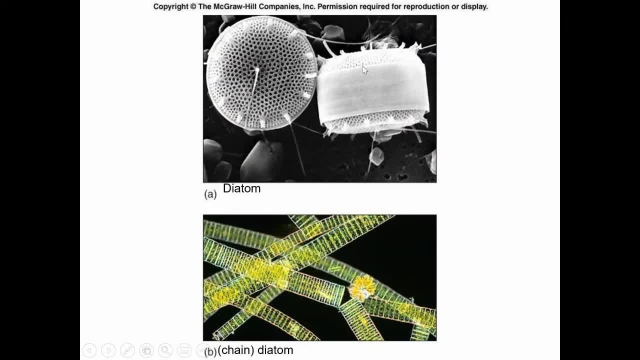 photosynthetic. Another classic shot of a diatom. This one helps you see the pancake idea: the two tombs stacked. You also see that they have all these little holes in them. That allows them to stay in the surface layer of the water column, because if they didn't again they'd fall out of the surface sunlit layer. 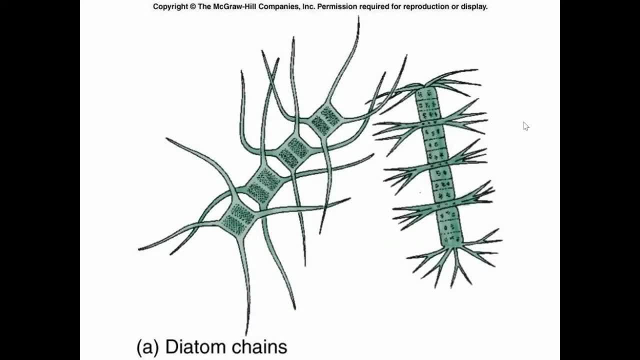 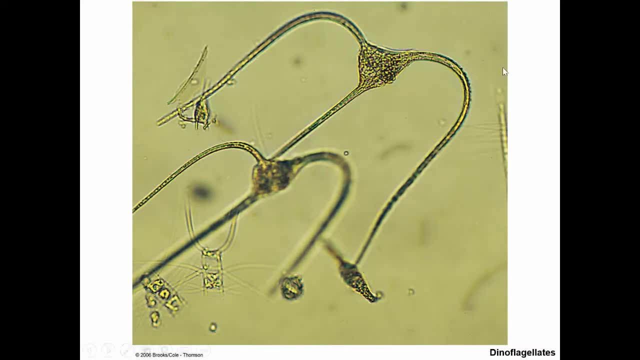 the top layer and they wouldn't be able to get the sun that they need. Another classic example is this guy here which is called a dinoflagellate. So a dinoflagellate is essentially that same stack little disc here, the diatom in the center, okay, But again, this is not a diatom, but it looks similar. 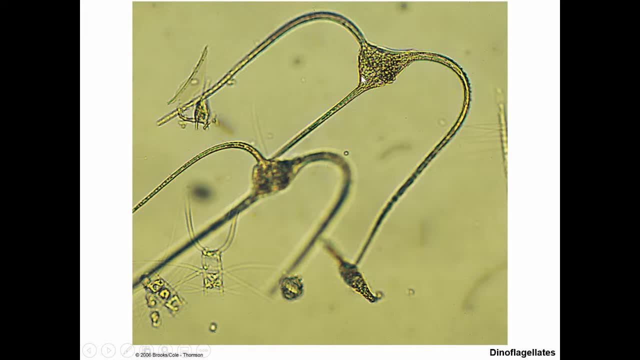 But then it has these whipped horns and this long tail. So its name, dinoflagellate, written right here for you. di means two flagella, two tails. This allows them to have mobility. They can actually move in the water. Now they're not swimming, which is why we still call them plankton, but just. 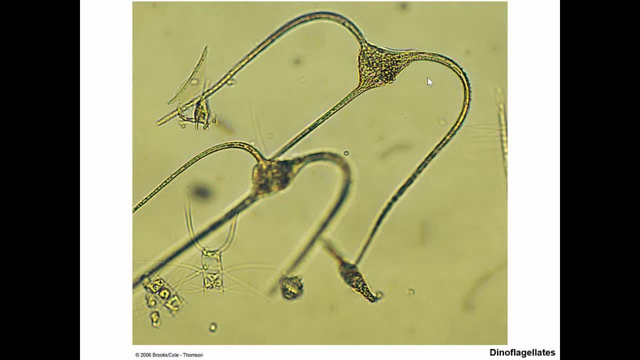 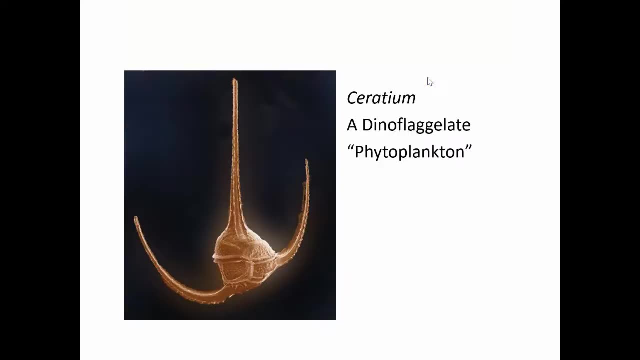 because they're plankton doesn't mean that they can't move at all. It just means they're so small and so light that they can't move at all. So they're not swimming, which is why we still call them plankton. but they can't fight the current, So they get the name phytoplankton, Some more cool. 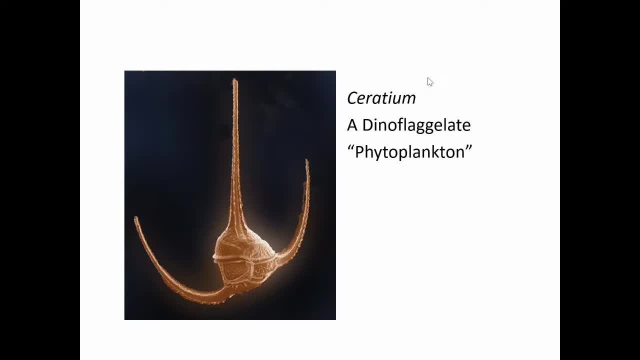 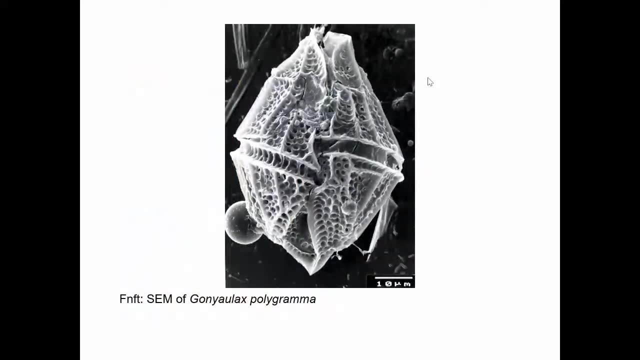 pictures of the dinoflagellates. These guys are the ones that cause the red tides that you hear about: mahogany tide, brown tide, green tide. Unfortunately, they can turn the water pretty polluted When there's a lack of oxygen or too much nutrients in the water. they can actually 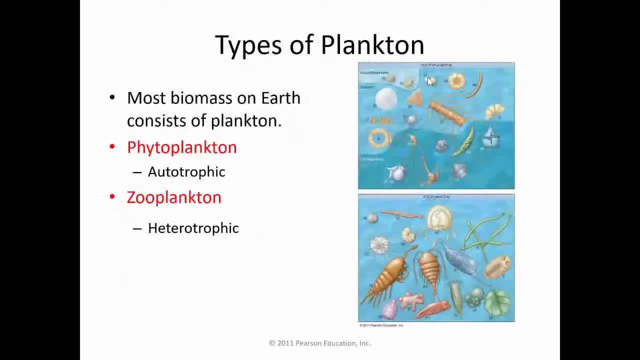 become sick, and then the water itself becomes sick. So these are just some really great pictures of phytoplankton. Now moving on to zooplankton. So where do you find animals in a zoo? So it's easy to remember animal plankton. Why are they? 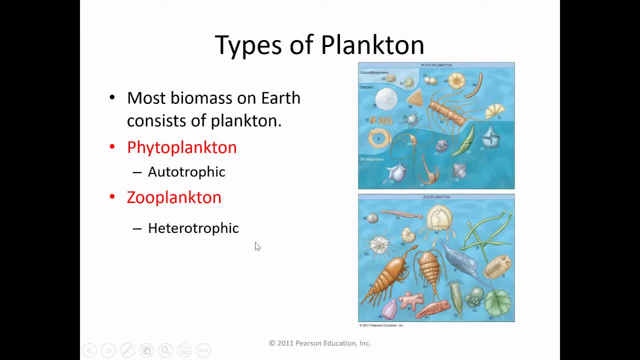 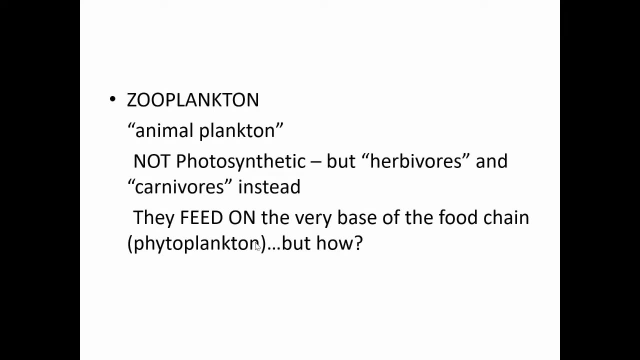 animals Because they're heterotrophic: They have to eat something else in order to survive. When we talk about zooplankton, these guys are not photosynthetic. okay, They're either herbivores or carnivores. Herbivores mean they are the first level consumer that feed on the phytoplankton. 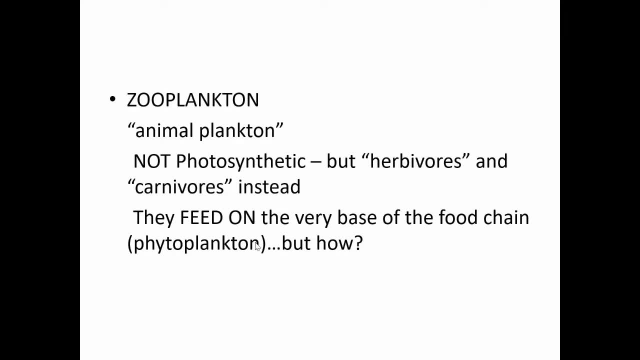 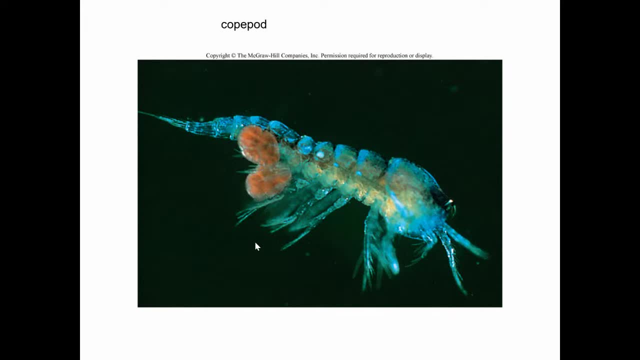 That's usually what happens in a juvenile stage, or they're higher level consumers. the carnivores on the second and third level of the zooplankton, The most populated right, the most numerous, is the copepod. Look kind of like shrimp, They're in. 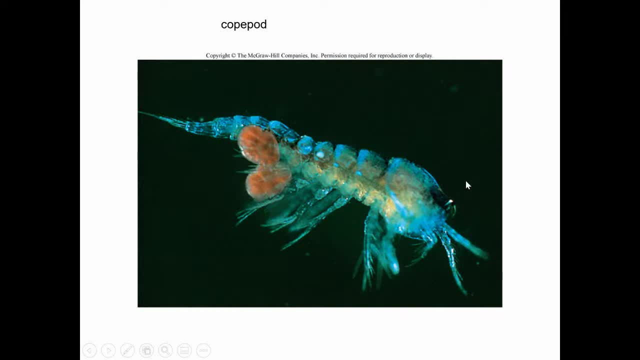 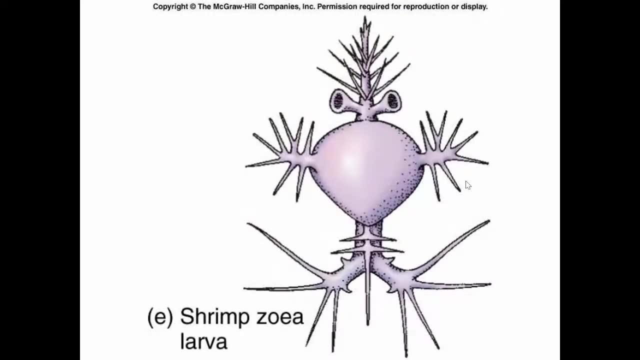 the arthropod classification. You see, they have these joint appendages along their body, but they're very, very prolific. Sometimes we study copepods in the ocean in order to determine their overall health. And again you saw all these cool life cycle images that crabs and shrimp and 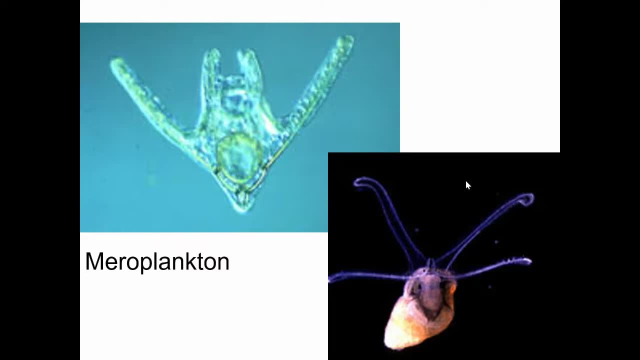 barnacles and lobster go through, But all of the marine invertebrates, almost all go through these invertebrates. So the copepod is a very prolific animal. So you see, the copepod is a very prolific animal. 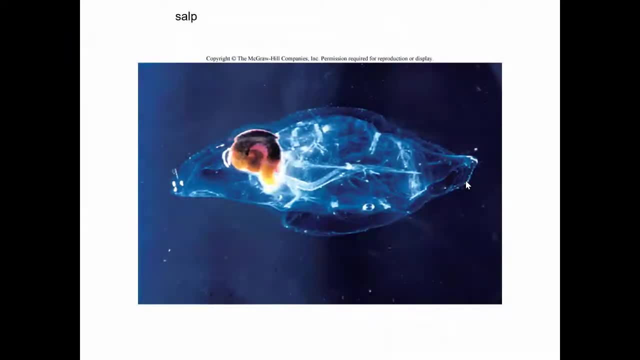 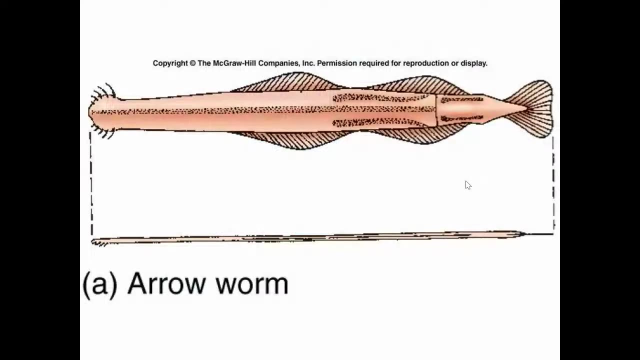 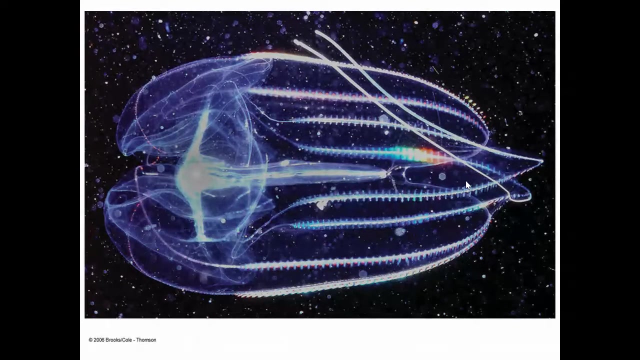 different stages. So here's a squid in its larval stage, a selp in its permanently planktonic stage. You have some turbularia and some different sea worms. You also have arrow worms, chetignaths, comb jellies. These guys are the ones that bioluminesce, Again large. You can see these. 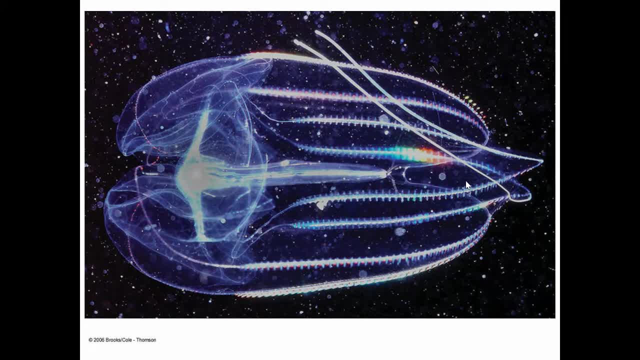 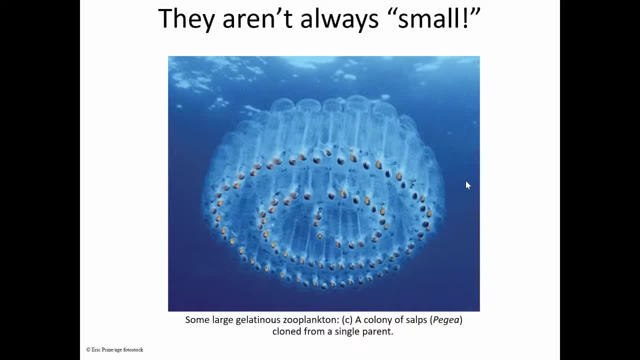 with the naked eye. These would fit in the palm of your hand, but because they can't fight against the current and swim, we classify them as zooplankton. Again reminder that they're not always small. Selps can gather colonially right collectively. The organism itself is here. 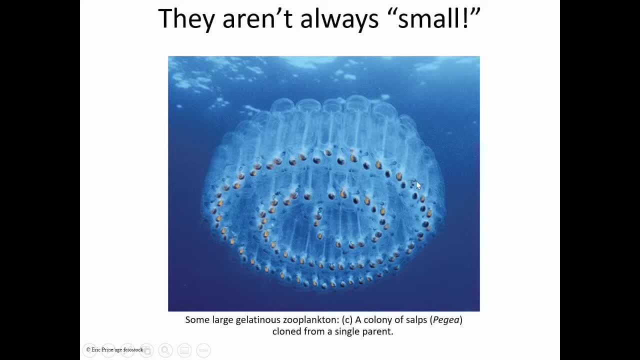 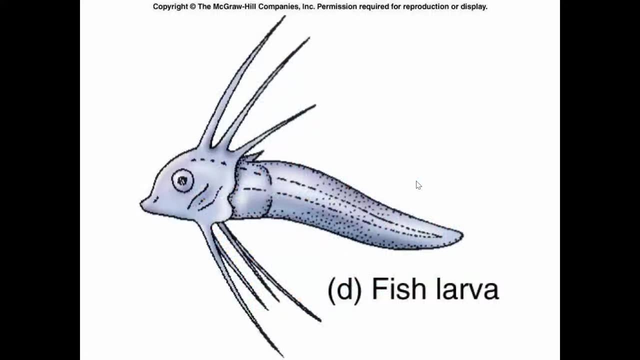 living essentially in this little house that allows them to filter feed- Pretty cool, And I like to use this picture to remind you guys that plankton doesn't mean small. Even fish, by the way, can end up in the zooplankton category. Most fish will then become large enough. 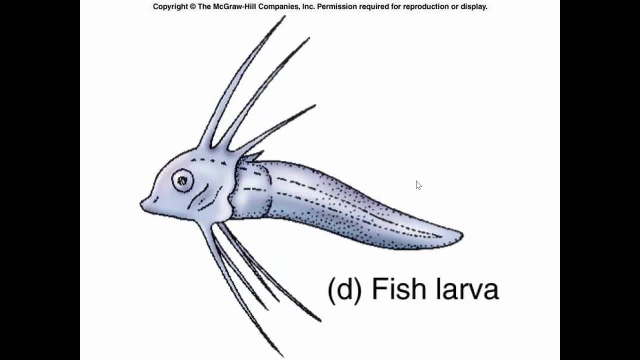 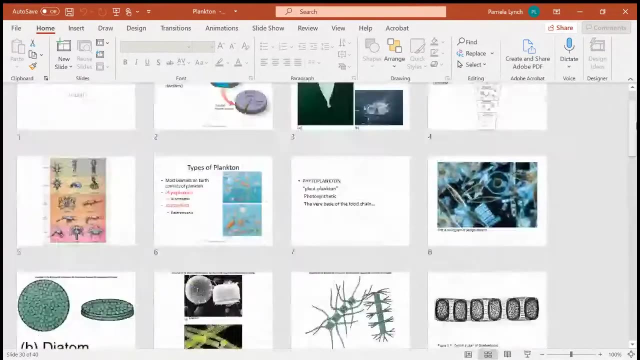 to either become nectin or benthos themselves. But a lot of fish, young-of-the-year fish, especially smaller fish, even in their adult stage, right, they end up to be really small and those fish start off in their planktonic stage. So just in summary, I want to remind you. 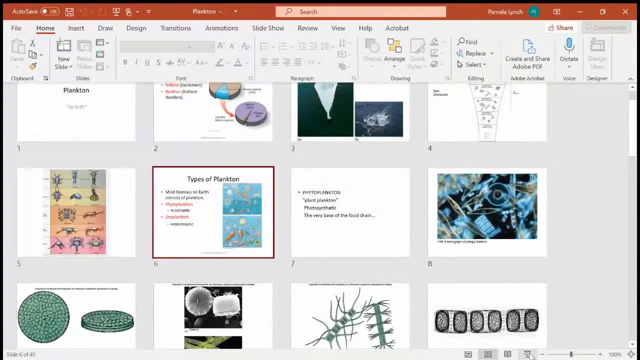 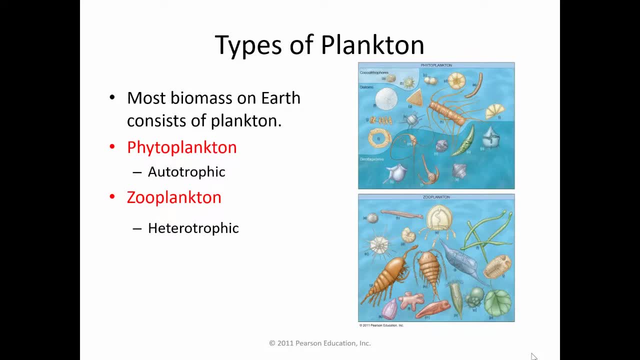 guys of the terms that I've introduced. okay, So we discussed what a plankton is. That means to float and drift. We highlighted the two different types: phytoplankton and zooplankton. Phytoplankton are autotrophic. 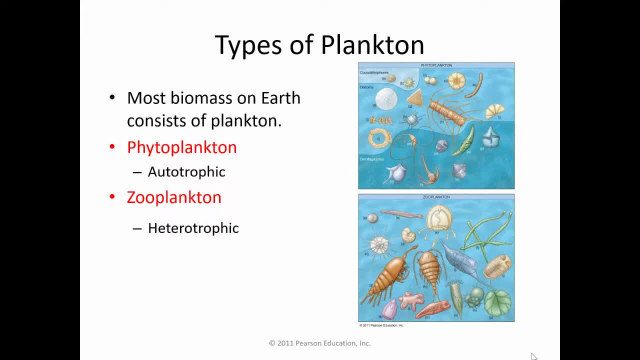 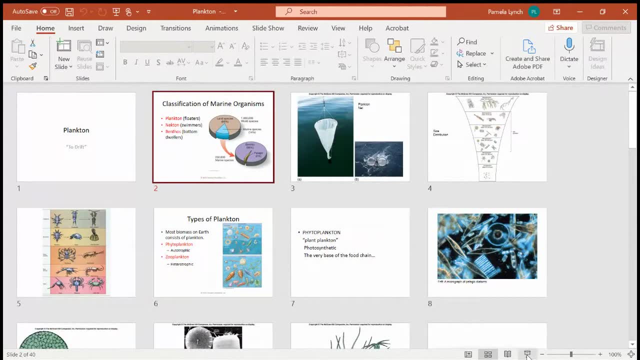 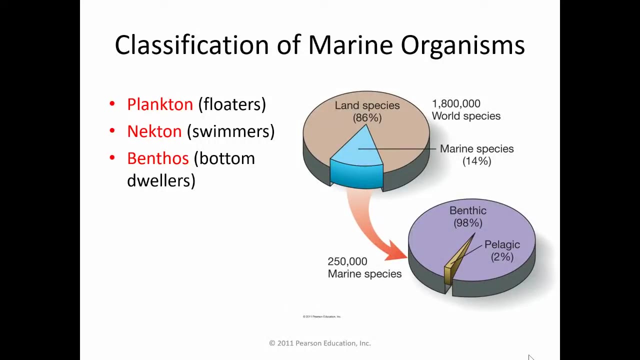 Zooplankton are heterotrophic, meaning producer and consumer. In addition to plankton, in the water column we also have nectin, which means to swim, And if you're not in the water column, if you're in or on the bottom, we call you benthos. So now I'm going to switch PowerPoints to the marine. 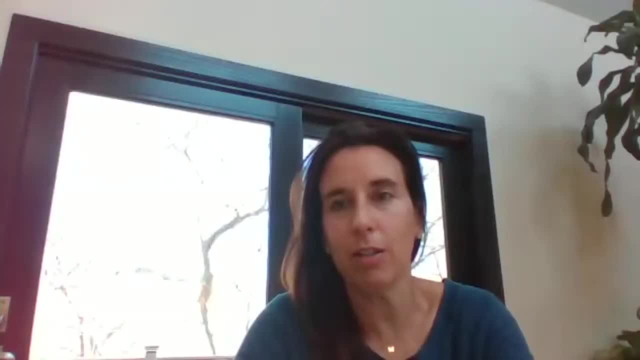 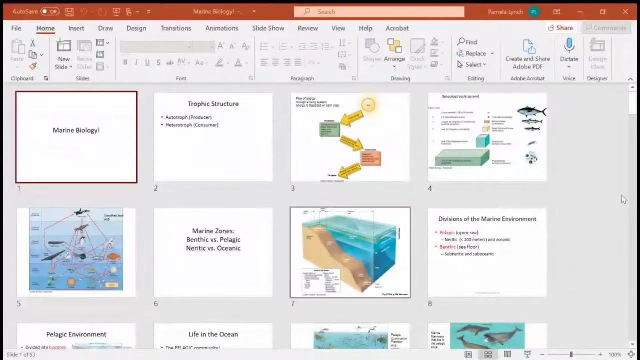 biology PowerPoint. Just give me a second here. I'm going to have to stop sharing this screen and then begin with a new screen, And if anyone on here that's watching has a hard time seeing any of this, please let me know. So now we're switching to the marine biology lecture. Everyone should see the marine biology. 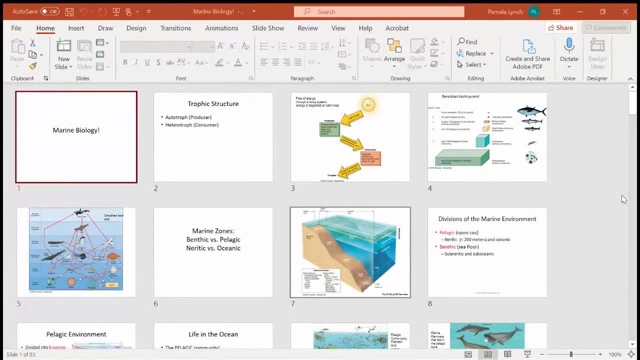 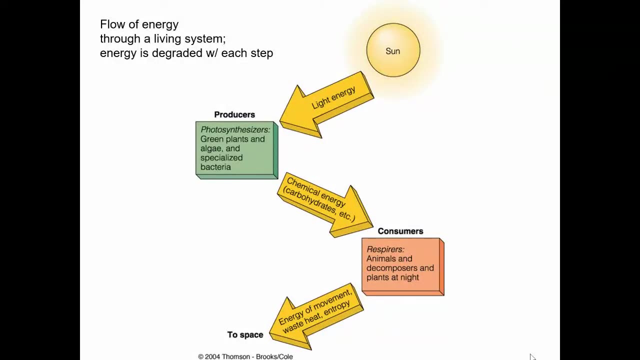 lecture now And you'll see that right away. it starts essentially where we left off right. We're talking about a trophic structure, We're talking about a feeding structure and introducing those really key, critical, important components of autotroph and heterotroph producer and consumer. So just quickly to remind you guys, 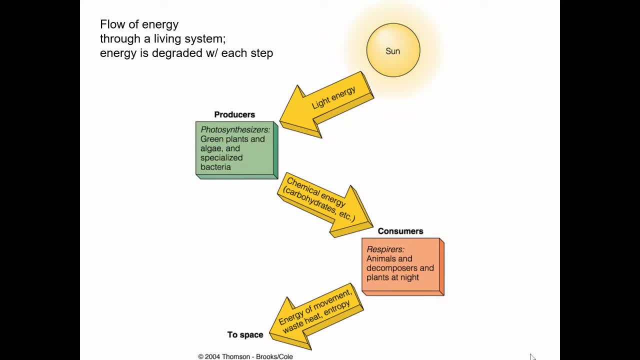 since we've talked a lot about the importance of autotroph and heterotroph producer and consumer, A lot about photosynthesis and the importance of primary production with plankton, that you guys understand the basis of how a trophic structure or a food web works in the ocean, By the way, 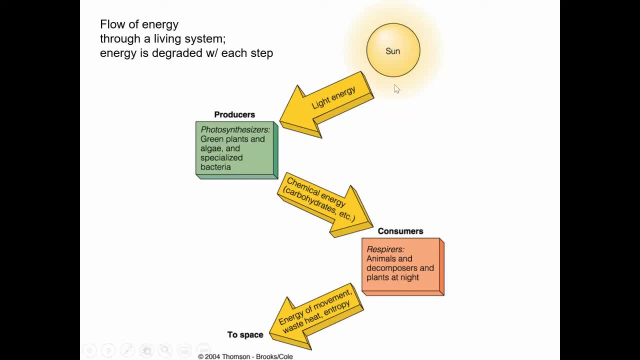 it works the exact same way in the ocean that it would on land. okay, So your sun produces light energy. Light energy gets absorbed by any of the autotrophs. It photosynthesizes In the ocean. that would happen with any seaweeds or algae, whether it be unicellular, one-celled algae. 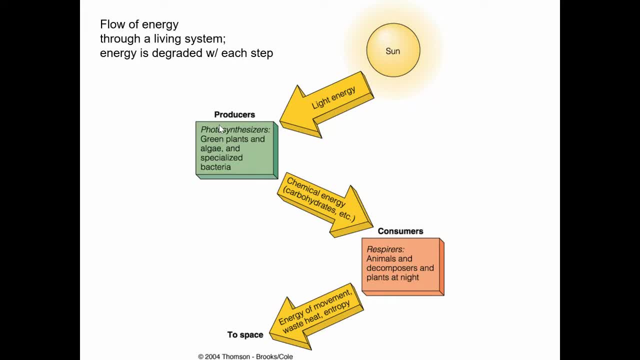 or multicellular algae, like a kelp, the stuff that's wrapped around your tuna roll when you go for sushi, Any plants like seagrasses, trees, like mangroves, and even some bacteria and specialized cells. Those are going to be all your producers or autotrophs. 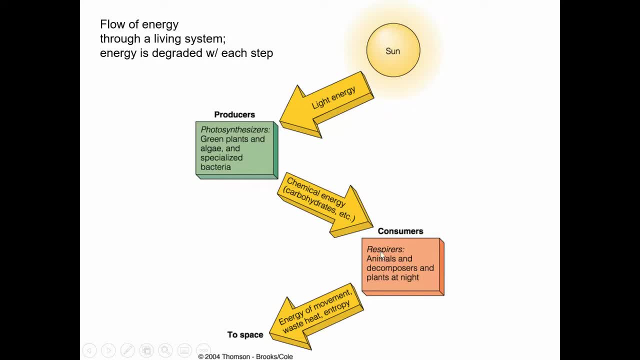 If they get eaten by something- here is your heterotrophs- the consumers then absorb that energy. They take in that food source. Those consumers then can get eaten by other, higher level consumers, So the energy just transfers up the food web. 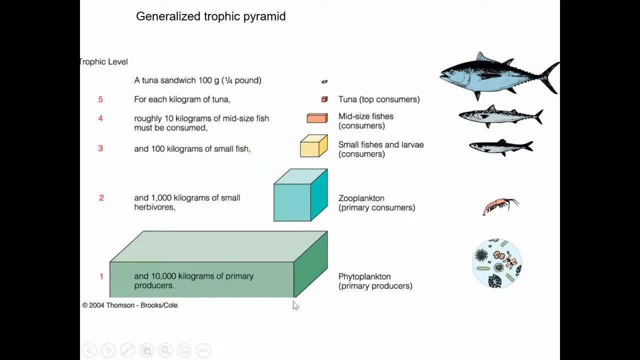 You're going to notice, and this is why I highlighted that plankton were so important from a numbers perspective. the lowest level, the base of the pyramid, the lowest level, contains the most. So the overall health of the ocean is extremely dependent upon the smallest microscopic. 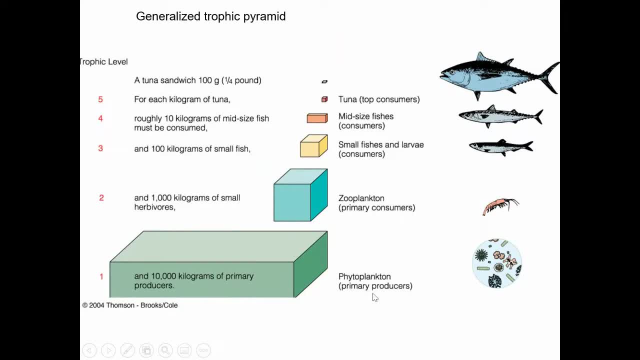 phytoplankton, the primary producers- those which you learned about in lab 10, of the ocean. It also, unfortunately, leads to pollution issues If the water itself is polluted and these organisms are living in that surface layer of the water column, and then they get eaten by these higher level organisms. 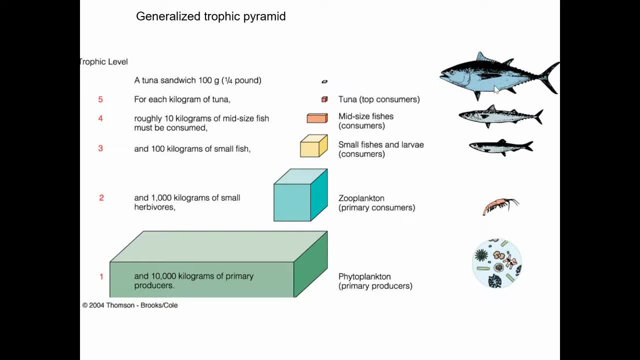 that material can accumulate or magnify- And often you'll hear that you're not supposed to eat a lot of mackerel or tuna if you're pregnant- or higher level trophic structure fish, because they have magnified metals or toxins, And this is exactly why. So, while the trophic structure, 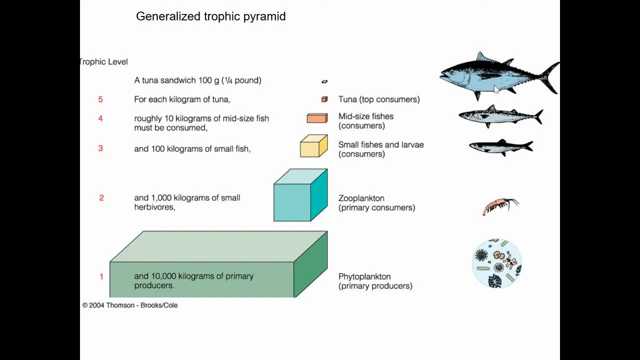 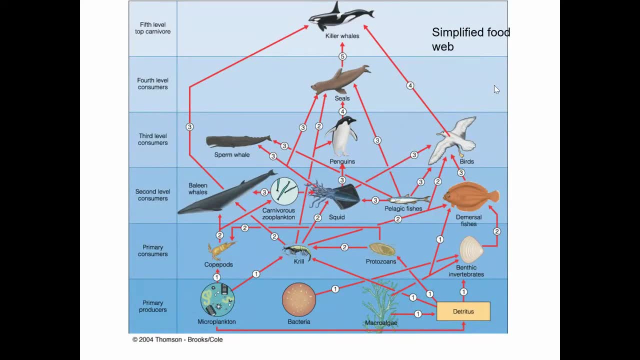 is amazing. it also can become dangerous if the oceans are unhealthy. Here's a crazy food web. gone crazy right Or gone wild. We like to call things not food pyramids or food chains. We like to call them webs, because you can see all these arrows right. All these arrows are pointing to all these different 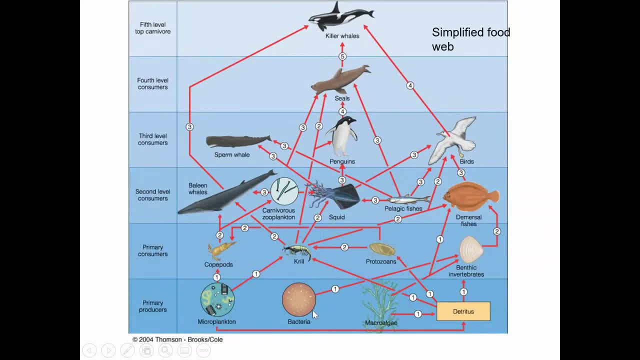 organisms. It means that multiple organisms exist on each level of the food web And I always say: if you go back in time and you step on a butterfly, do you change the world? Well, if we pulled the squid out of this food web, would we change the web? 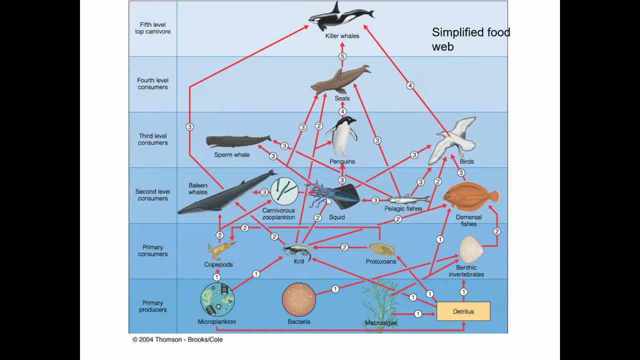 Yes, right, Each and every living thing on this planet is the food source for something else. Even in its death, even the waste it produces can be a food source for something. The actual food web is extremely complex and very, very, very high quality, meaning there's. 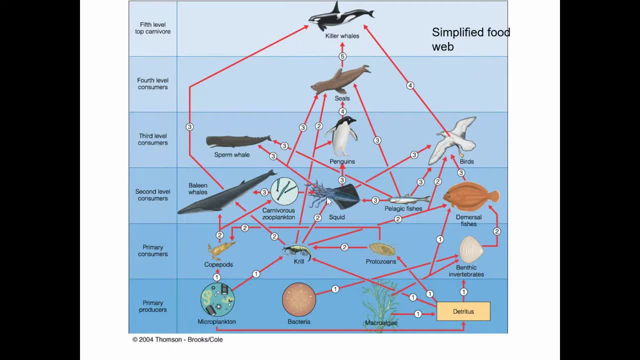 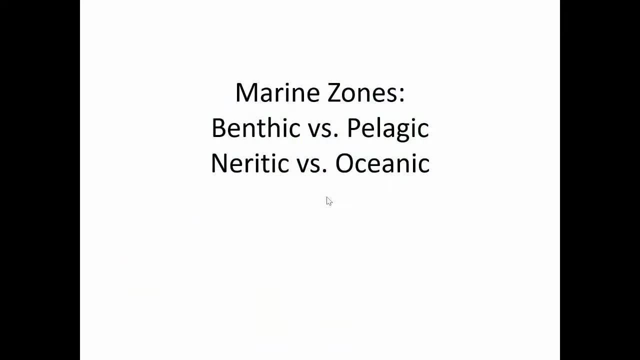 so that each of these organisms can maintain their component, maintain their structure on the food web. Okay, so that's my introduction to plankton as a whole and, of course, food webs and the concepts between autotroph and heterotroph. When we introduced the word plankton, we then gave 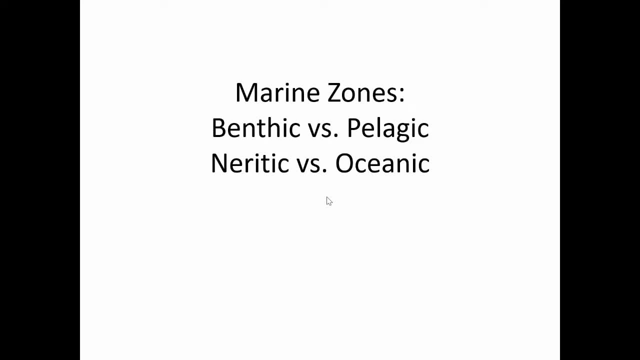 the description of it being plankton as floating and drifting, or nectin as swimming. We said that it was a very complex and complex food. It's not something you can find anywhere else, So we're going to go through it. So we're going to go through it. So the first part of the course. 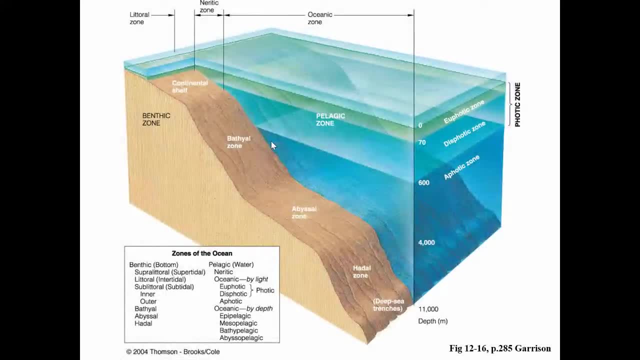 is in the water column. Okay, so now what I'm going to show you are the terms for those areas in the water column. Remember, we already learned benthos, right, But we're going to learn a couple new ones. So now, from an oceanography perspective- you guys are used to this word, right? Think all. 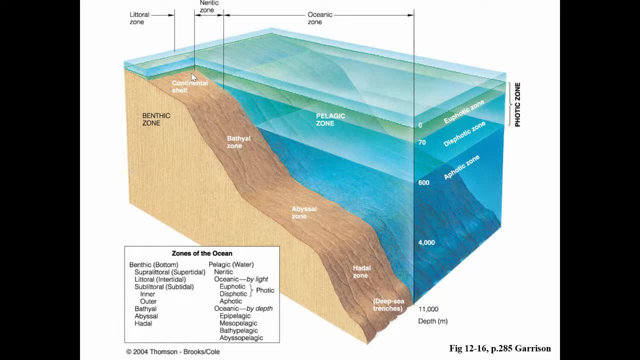 the way back to section one of the course. You know what a continental shelf is. We talked about the continental margin, Remember. the margin is the edge shelf extends to this line here where our shelf break would be. then we would have our slope and 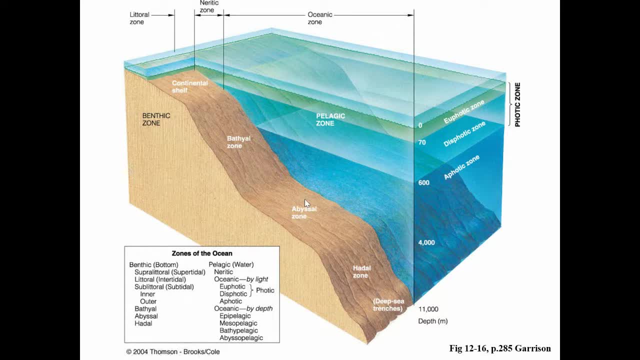 our rise until we get out into where the continental crust switches over to the oceanic crust. Now, from a marine biology perspective, we then have to realize that that brown stuff, that earth, that rock, whether it be granite or basalt, is covered by water and is the home of. 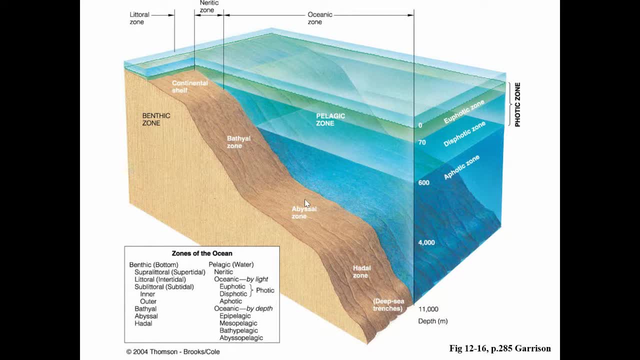 organisms. Things live in the bottom. on the bottom, Things are living in the water and moving back and forth between them. So, instead of using continental shelf break, slope and rise, or even continental margin as a term, we instead use the words benthic and the organisms that live in the. 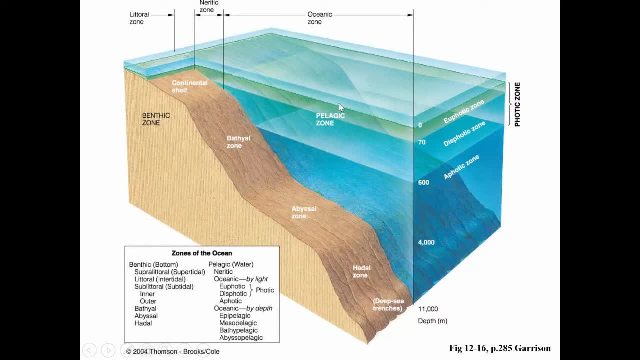 benthic are called benthos and pelagic. Pelagic again would be a new term here. Okay, this means any of the blue on the picture, blue in the water column. The pelagic organisms are the two that we just described. So we have the blue in the water column, the blue in the water column and the 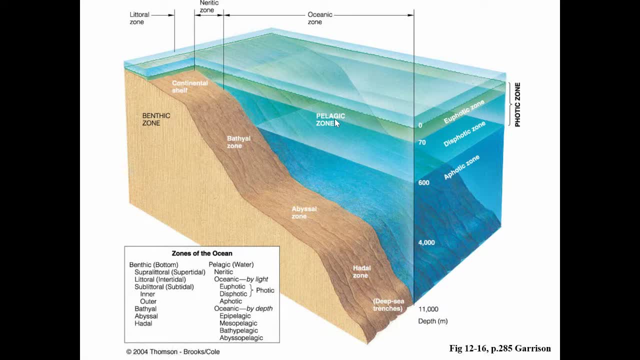 blue in the water column. So we've already covered plankton. I want to use the rest of this lecture to introduce you to the nectin and the benthos, paying particular attention, of course, to some of the actual habitats, actual structural habitats as well, So not just organisms singularly. 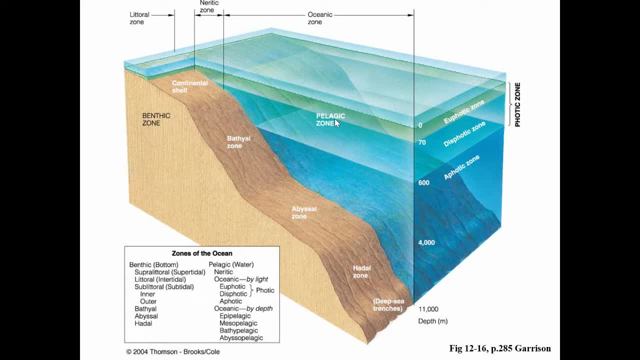 but those that live together in very specific communities. You'll also notice on this picture that it shows you that the ocean can be deep. as we know right, The Mariana Trench starts seven miles down, So of course there's a lot of different deep spots. But what does that? 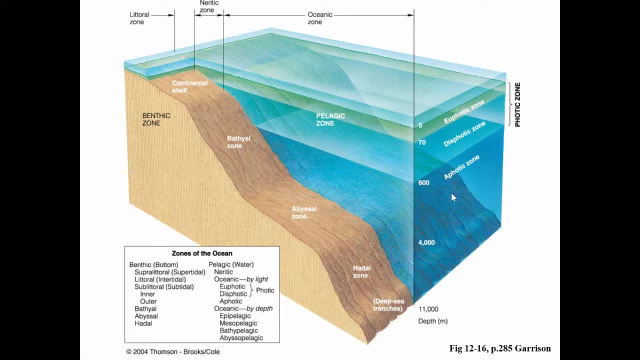 mean from a living perspective. What does it mean if you're a primary producer, that which needs the sun to make sugar? Well, it means you need to live in the surface layer, right? We call that the photic zone. A photic zone means there's sunlight. Anything below the photic zone without light, a photic. 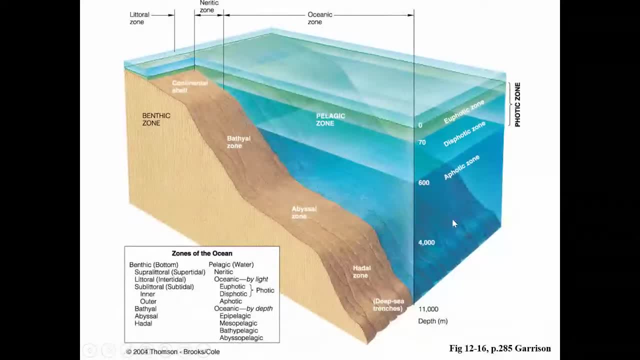 zone. this can't have primary production. This cannot have phytoplankton living in it. They can be dead and falling through the ocean. So if you're a primary producer, you need to live in the surface layer. You can't have phytoplankton falling through the water column to be a food source for something on. 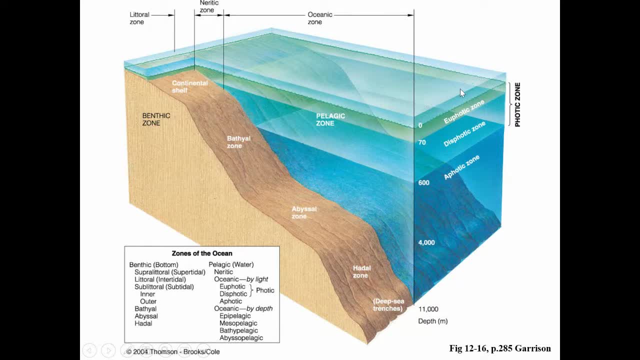 the bottom, But living phytoplankton have to live in the surface layer. Zooplankton, conversely, can live in any water column. Most of them live right below the very, very, very top of the water, in the euphotic zone, because they want to be just underneath the phytoplankton so that they can feed. 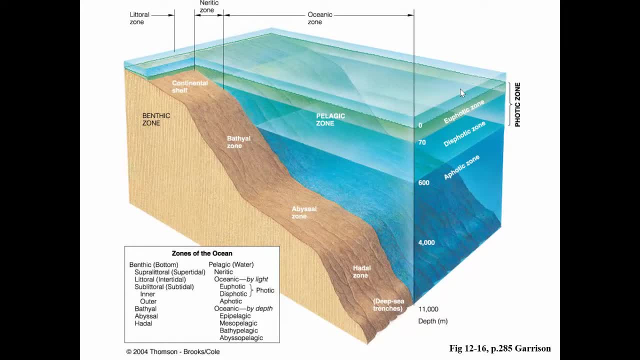 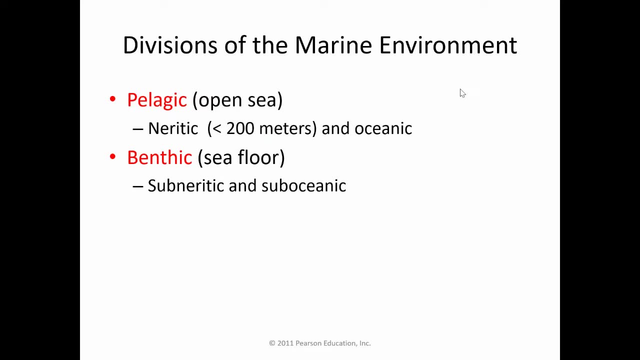 on them. But again, because they don't need the sunlight, they can live in any water column. So just a reminder of what those key terms are. Okay, so we have the pelagic area. That's where the water is, That's where your plankton and your nectin are going to be. 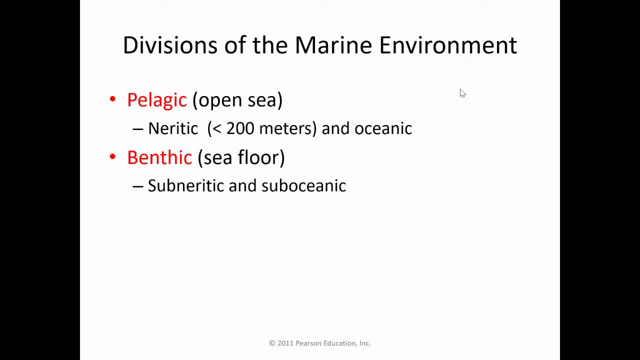 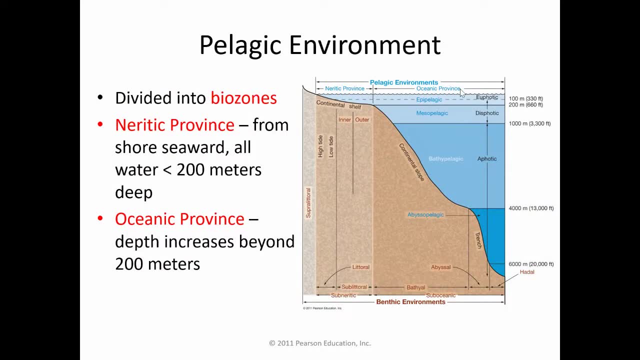 And then we have our benthos. Benthos are going to be that which is on the bottom or in the bottom. Here's another shot of the same thing. Remember, there's all different views whether you have an active margin or a passive margin. right, if your shelf is going to be. 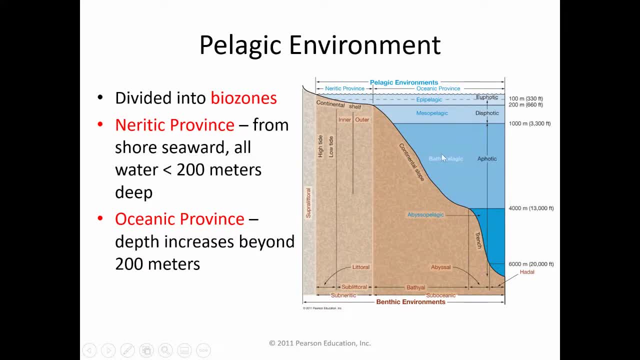 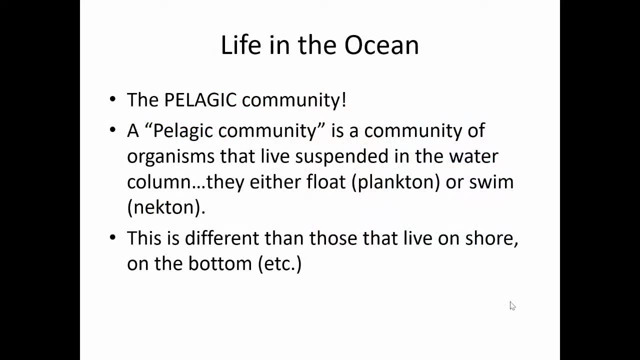 narrow or skinny. It also shows you that the different layers produce or have the ability for sunlight to penetrate or not. Okay so let's take a look at some organisms in the pelagic community. Okay so, in the same way that we looked at plankton already, we already know the 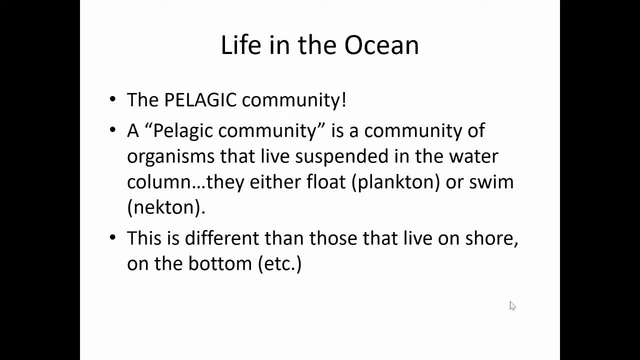 plankton are there, Okay? so we looked at a bunch of cool pictures of diatoms and dinoflagellates, And then we also- those were your phytoplankton- And then we also looked at a bunch of different zooplankton. But what about some nectin, right? So let's look at a reminder of all that stuff. 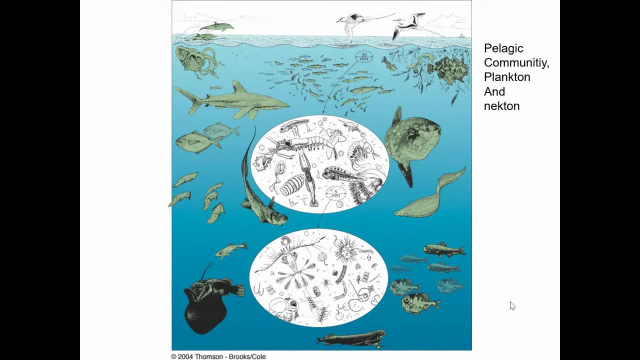 that's going to be in the water column. Well, here's just a beautiful cross view, or a cross shot of all of that stuff that you can see. These white dots are supposed to represent what you would see under a microscope, right? So that represents the plankton. 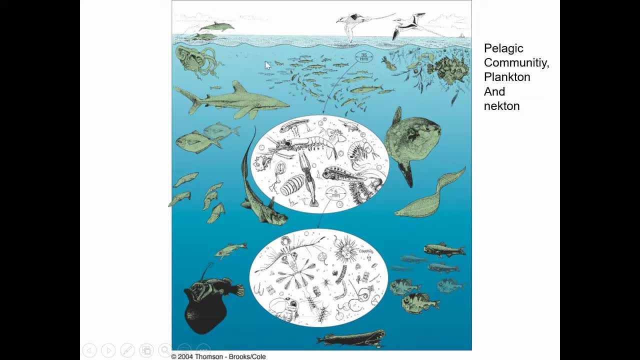 We already covered. But what else is in the water? Well, of course, in the surface layer of the water, you're going to have all of your migratory fish that are going to be at the surface because they need to feed on the plankton that are there. You're also going to have some mammals. 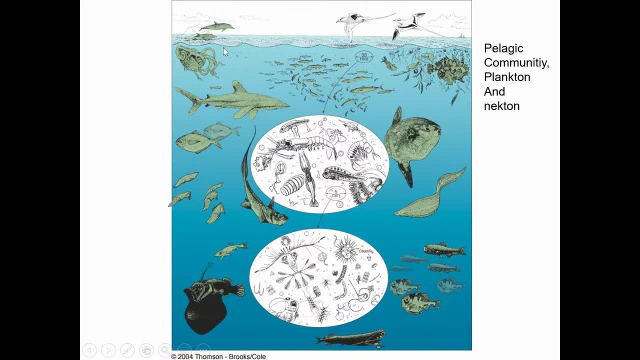 represented here by some turtles and some birds, all of which that are living in that very surface layer of the water column, because that's where their food source is. As you drop deeper in the water column, you'll notice that the types of organisms that you find, like this anglerfish- 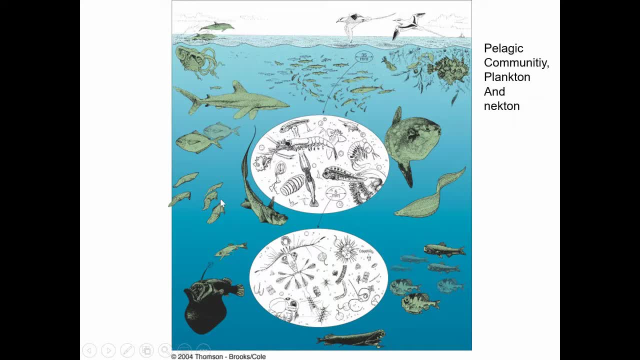 become different. Organisms have different structural abilities, different physical characteristics, essentially to be able to live in the environment. Think about what you know from oceanography. If we are way down in the water column, what's going on down there? It's pitch dark, It's freezing. 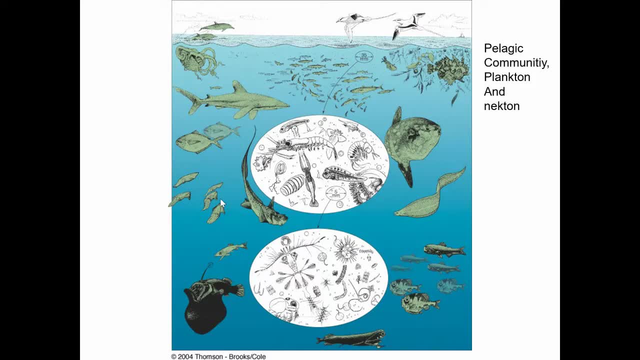 cold. There's a lot of salinity, There's a lot of pressure. So if you're an organism that lives there permanently, you have to handle that harsh environment. If you're an organism that can't, you're going to be living in the surface layer, and vice versa. 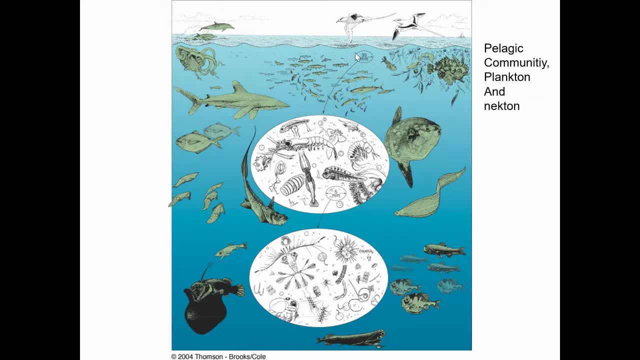 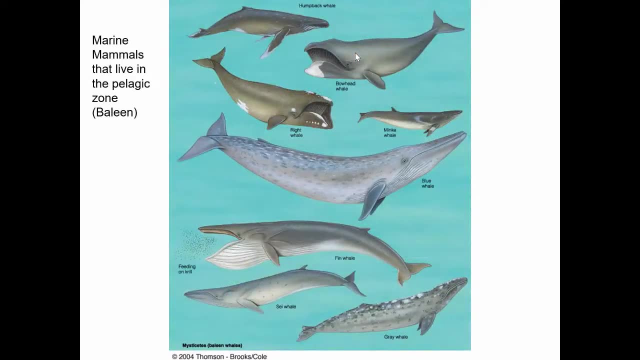 So what it does is it has different types of organisms living in different parts of the ocean, based on what types of water quality or habitats that they can withstand. So, of course, in the surface layers for migration purposes, we find all of our whales- Whales. 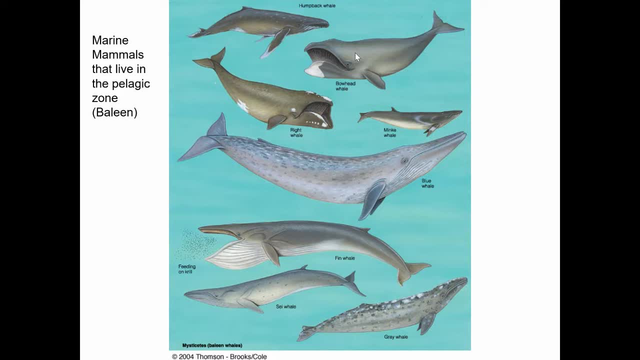 though, can dive down up to a mile deep, because their food sources- and again, not all of them, right especially sperm whales, love to dive down. because their favorite food source is the colossal or the giant squid, They like to come to the surface for mating purposes and for migratory purposes. When we 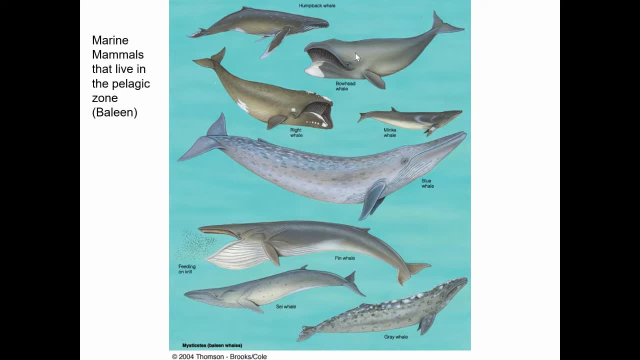 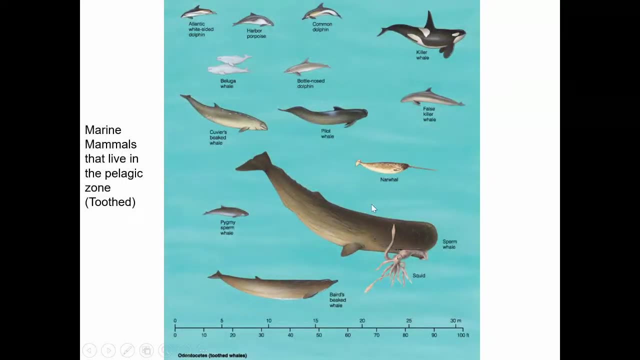 think of whales. you guys need to realize there are two kinds of whales: Those which you're looking at now in this picture, which are the baleen whales, and those which you're looking at in this picture, And here's the sperm whale fighting with the giant squid. These guys are toothed. 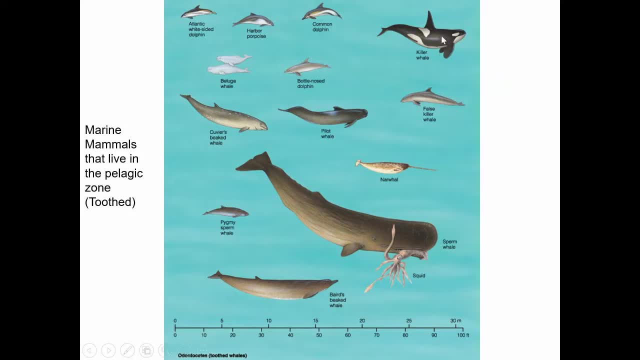 whales or the odontocy. probably the most famous of all is Shamu, the killer whale, But many of you probably didn't even realize that a dolphin or a porpoise is a whale. Narwhal unicorn of the sea- another really cool whale. But what you're noticing is that even the 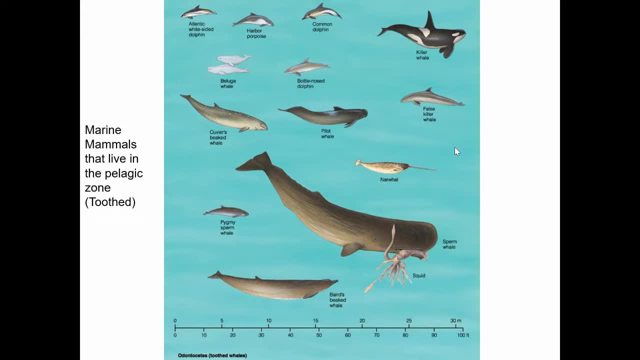 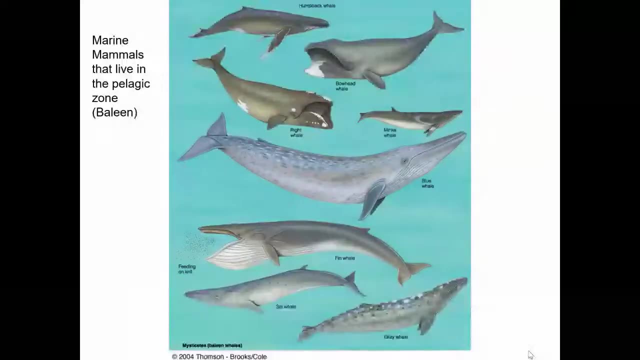 whales have different physical capabilities. right The way that they feed is totally different If we go back and we take a look at those baleen whales. baleen whales means that they filter feed. They have a mouth made essentially of like this: upside down like broom, It's like a very 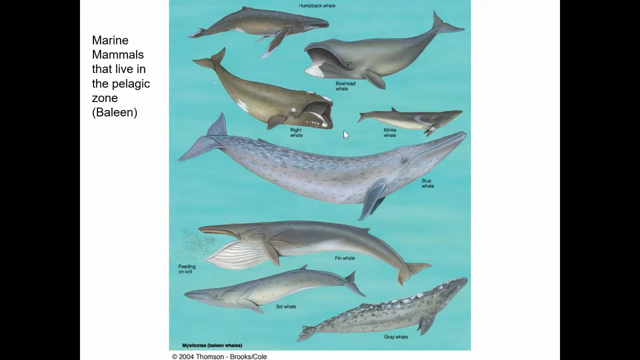 very thick, coarse, giant toothbrush hanging from its mouth. So when it swims it swims with its mouth closed, but it's open right, Because water can go through This toothbrush. So what do you think gets stuck in there? Plankton, The largest animal on the. 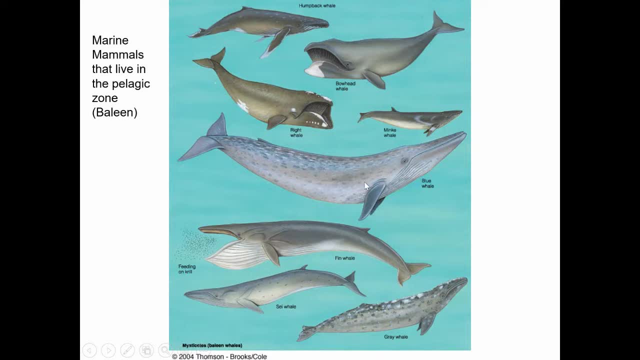 planet. the blue whale feeds almost exclusively on krill, which is a zooplankton, one of the smallest animals on the planet. So here we are with that link, Here we are with that food web that highlights that saving the whales literally means saving the plankton first, because you can't 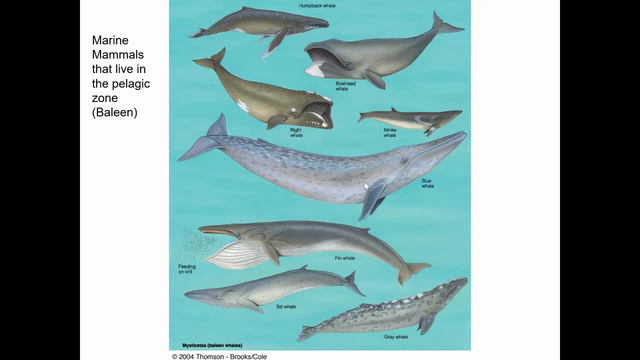 take their food source out. And when you actually when Greenpeace and all these other organizations, scientific organizations, non-profit organizations- when they want to survey the health of a whale, they actually survey the krill, Because if there's no krill in the water, it doesn't matter. And so now hopefully, you're starting to see that, while 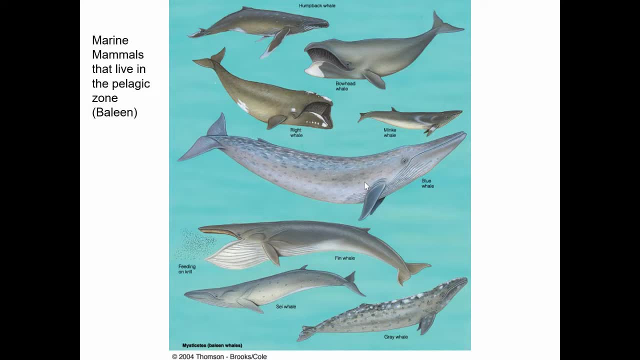 these are the charismatic megafauna. these are the cool things we like to look at. the stuff we really should be protecting and focusing on is the water quality itself and the plankton within it, because they become the base of the food chain for all of our biggest organisms. 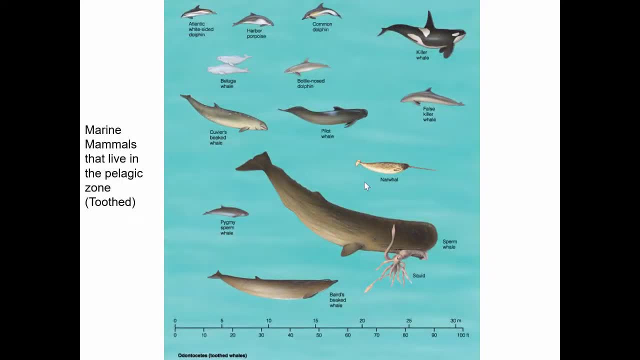 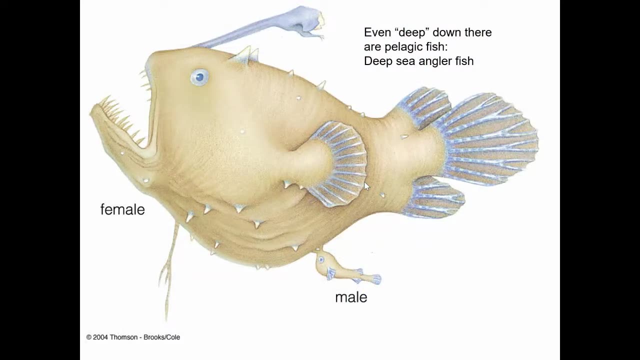 So whales, of course, are a great example to study in marine biology. There's also some really cool again, as that picture has shown you. there's stuff in the surface layer of the water column and then those which are found a lot deeper in the water column. Anglerfish have these. 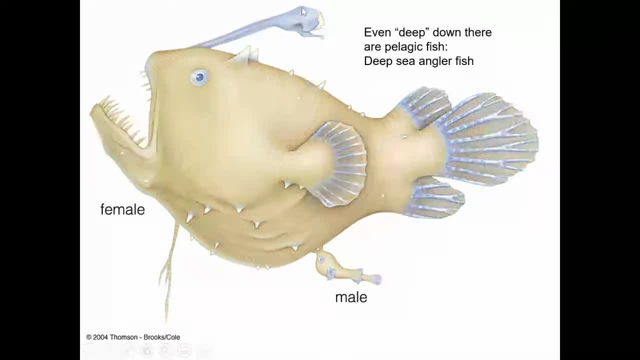 really cool capabilities of having bioluminescent lures, stuff that lights up and flashes. This will essentially get hung in front of its mouth with these giant teeth and the lantern will light up and then prey will come and say: oh, what was that flash in the dark? right They're. 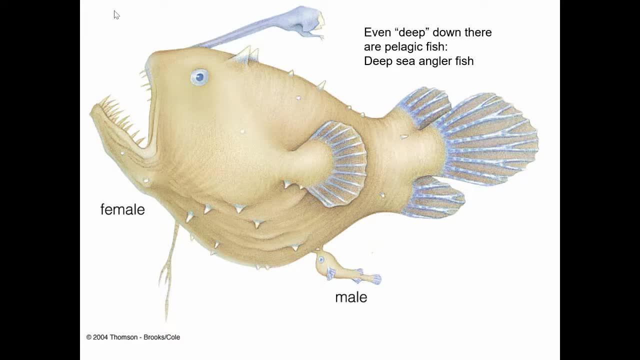 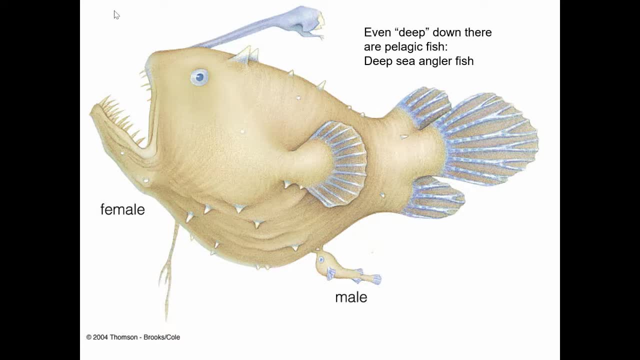 is sitting right in front of the mouth of the fish. Most of you have seen this in Nemo and other marine cartoons and things, but it's a really cool adaptation that this particular organism has. They also have some really cool mating techniques, So this picture shows how the 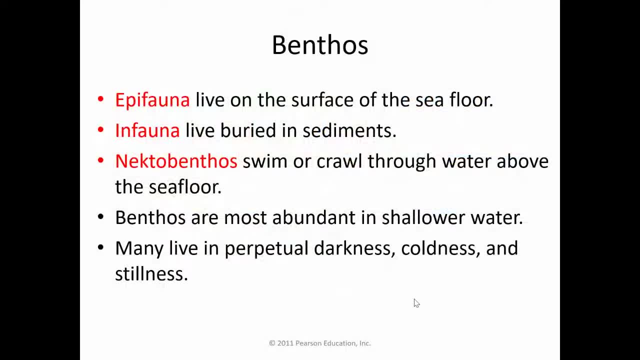 male attaches to the female for permanent production. So those are some classic examples of nectin, right? So we talked about plankton. Those are just a few about nectin. And now I want to touch and remember: those are in the pelagic or in the water column. I want to 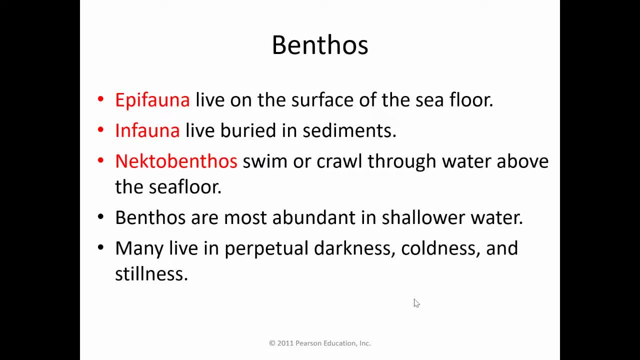 touch now on the benthos. Benthos means benthic, Benthic means that it's an organism that's in or on the bottom. okay, So you can live permanently attached. you can be buried in the sediment or you can swim directly above the seafloor but then land on the seafloor for feeding. 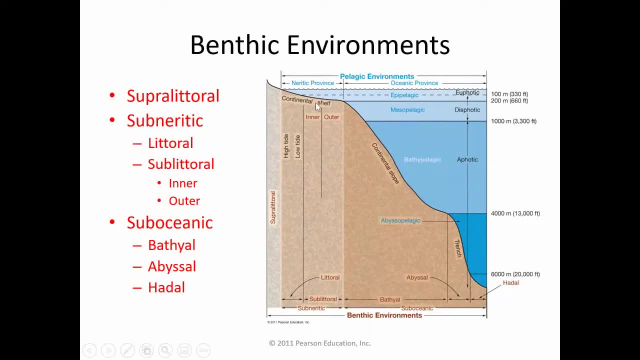 So benthos supports a ton of different organisms as well. In this picture that you saw already, it means you would live anywhere along the seafloor and you would live anywhere along the this line- okay, In it on it, hovering above it, or even being in the water column and then landing. 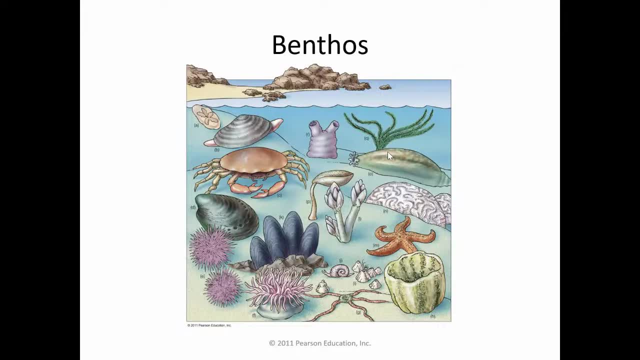 on it temporarily. So here's some classic benthos: those which are permanently attached, like mussels or barnacles or a giant clam or a coral. Those which can cruise around like a sea star or a brittle star or a sea urchin or a crab. Those which can burrow in like a surf clam, right. 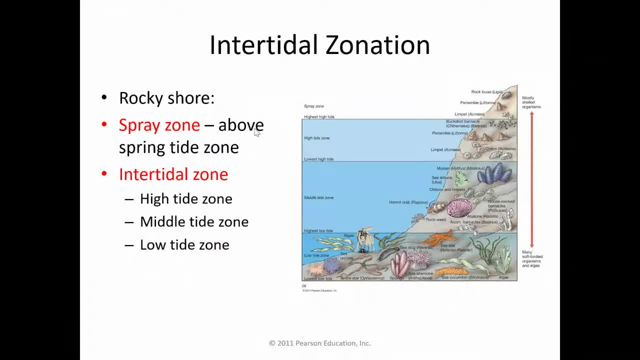 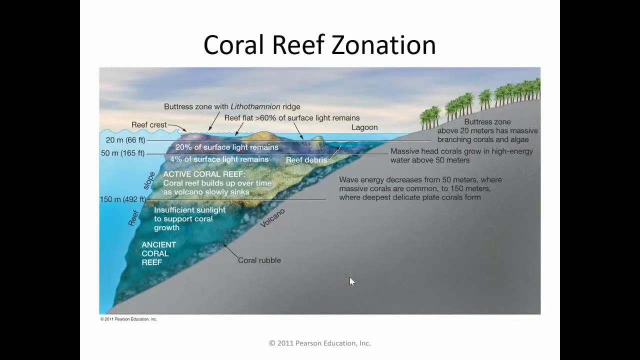 So there's all these different examples of what benthos can mean. Benthos, of course, can be right in the intertidal zone and extend all the way to the deepest, darkest depths of the water column, So the entire ocean floor is littered with life. The most famous of all of our benthic habitats is 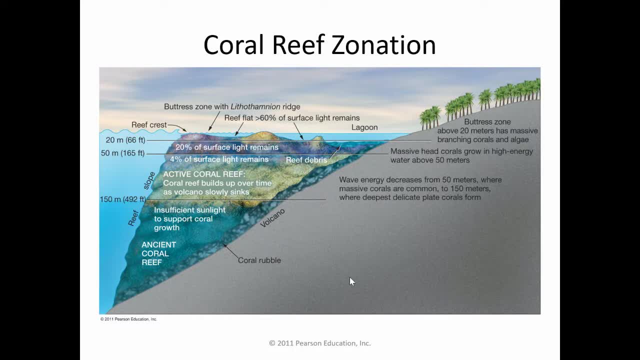 coral. They form a reef system. Unfortunately, there are less than one percent of all living coral reefs left on the planet. So there are less than one percent of all living coral reefs left on the planet. Because the oceans are warming and because the oceans are polluted. Corals, as you can see, are 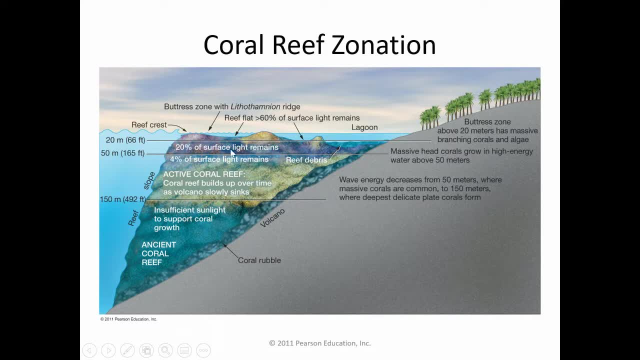 very close to the land. right, They exist in the epipelagic and in the epibenthic zones. Epi means surface, So they're in the surface layers and extend only to about two, three hundred feet. right Why: Coral reefs contain plankton, phytoplankton. You know phytoplankton need to. 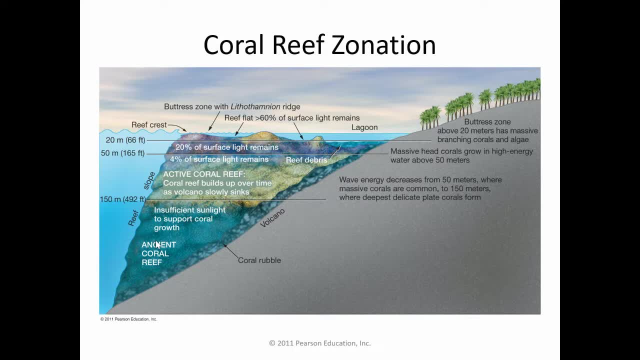 photosynthesize. So they're in the surface layers and they're in the surface layers and they're in the. So corals can only exist in areas of the ocean that have sunlight. They only can be in that photic zone. There's only so much photic zone that can be attached. They also because they're benthic. 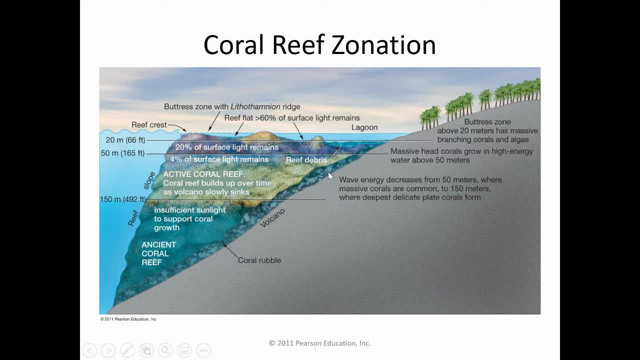 have to be attached to the side, essentially, of the rock, And so they become a living structure, a living reef, a rock filled with living organisms. Coral reefs become the most famous of all of our benthic habitats, And they also are the ones that need the most protecting. 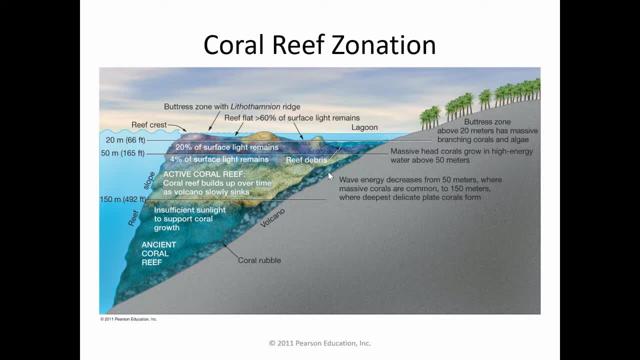 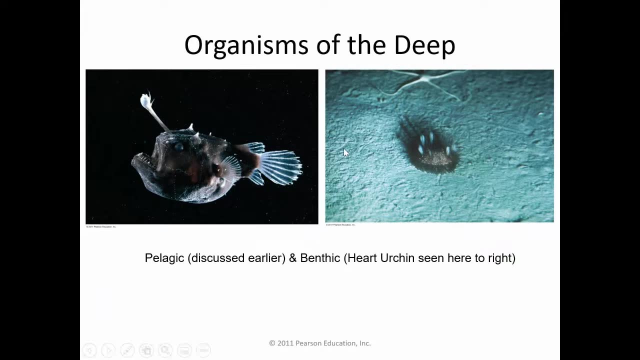 Kelp forests fit in this category As well. instead of being in a tropical zone, like a coral reef, kelp you typically find in a temperate zone. So just to highlight that, even in the deep areas, right? so we just mentioned that, of course. 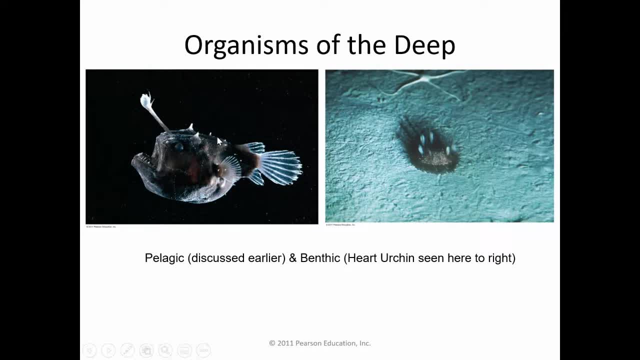 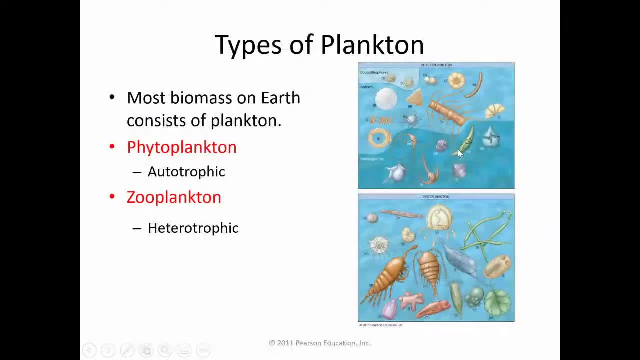 there's benthos in the shallows, but there's also benthos in the deep. Here we gave a nectonic example. There's our lanternfish. Here becomes a benthic like a heart urchin. Let's just highlight. 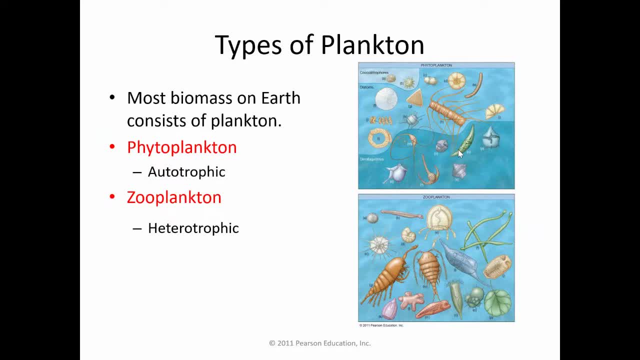 one more time, sort of in summary format, the different types of life. So we can do a general survey of marine biology. We can do a general survey of marine biology. We can do a general survey of marine biology in the ocean. Okay, so, starting first and foremost, I can't say enough about 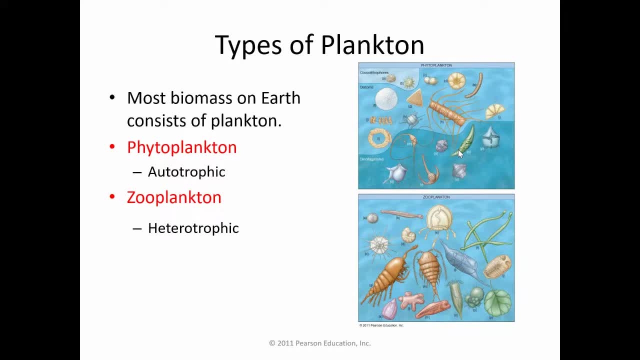 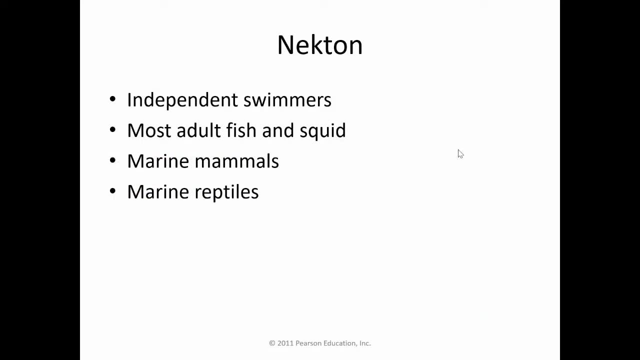 plankton right. Plankton are going to be one of the two examples of those which live in the pelagic area. Plankton are phytoplankton and zooplankton, The nectin the swimmers become. 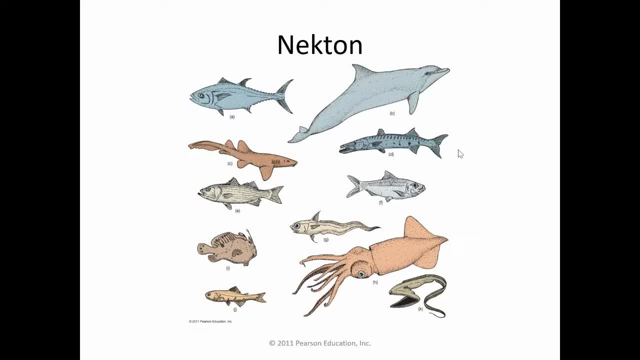 everything else. Those are that which can swim against a current. They include fish, They include reptiles, They include birds, mammals and invertebrates as well, represented here by the squid. Again, if you have a nectonic, you can do a general survey of marine biology. You can do a 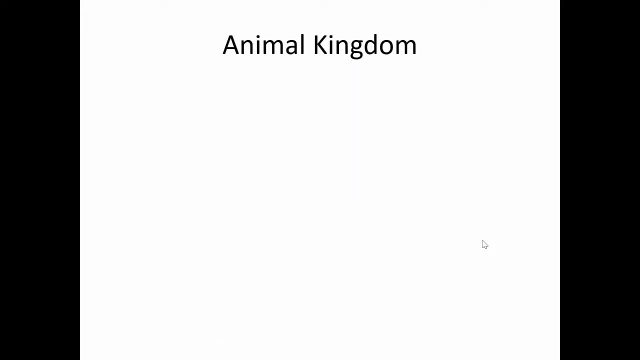 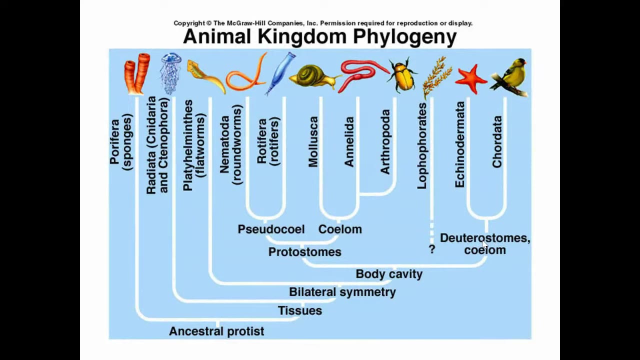 general survey of marine biology. You can do a general survey of marine biology. Invertebrates can start off as plankton and then become nectin. So what I would like to do, let me just fast forward here for a second. There we go. What I would like to do is, for about 10 minutes or so, just a general 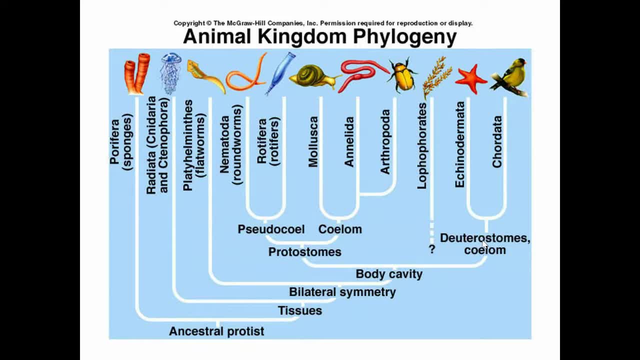 survey of life. okay, I don't want this lecture to go too long and the point is not for you guys to memorize the different kingdoms in the animal- excuse me, the different phyla in the animal kingdoms, but it's to recognize that we have a vast diversity of life in the ocean. 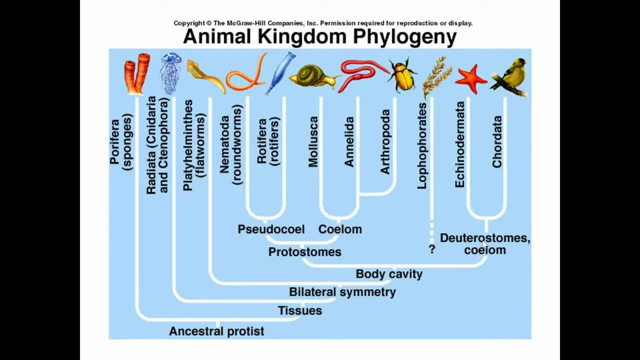 We, of course, have a vast diversity of life on land, and this particular phylogeny or family tree right, shows marine organisms, but also terrestrial organisms as well. Life is life, Whether you live in the ocean or you live on land you all ascended from and descended from. 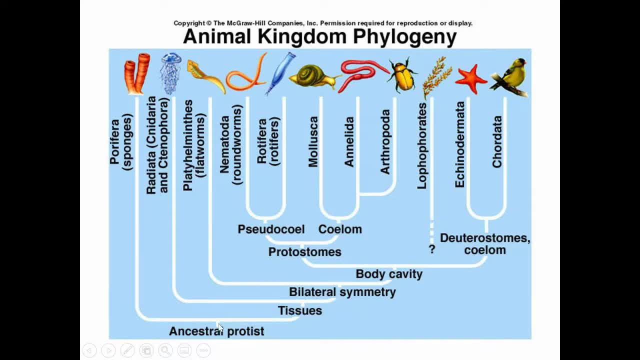 the same common ancestor. It's called a leuca, the last universal common ancestor. That's right here listed under the protists. We then evolve or change over time to form different structures, different body capabilities, In the same way that that lantern. 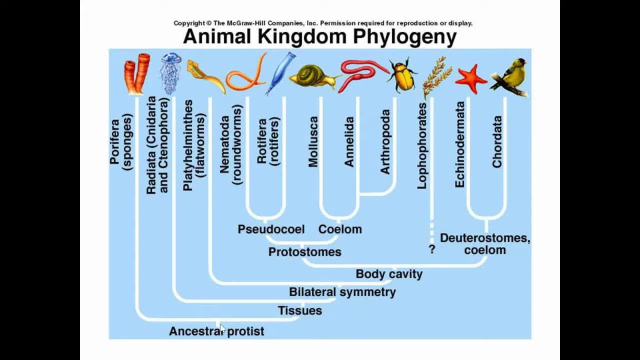 fish needs that lure to collect food, and I wouldn't, because I don't live in a deep, dark ocean. each organism needs different stuff to live and be successful in its role. A bird needs to fly because it lives in trees, nests in trees, mates in trees and hovers over the ocean to feed on. 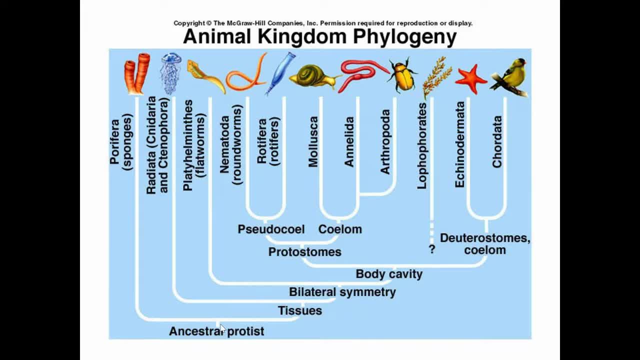 fish or hovers over the forest to feed on bugs. A snail doesn't need to fly because it's benthic right and it's feeding on different things. So you can see that a beetle is totally different than a sea star, is different than a bird. 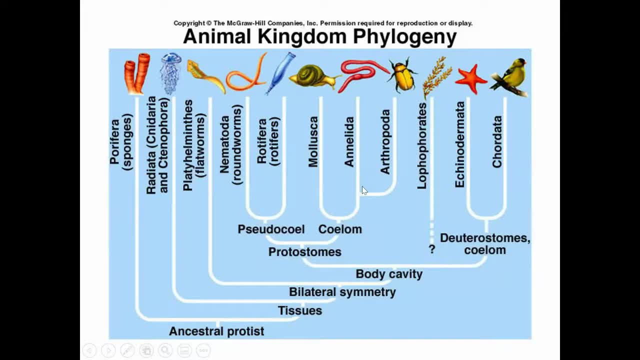 is different than a jellyfish: Diversity. Diversity is key in the ocean, just like diversity is key on land. So I just want to spend again a couple of minutes introducing you to the cool diversity of the animals in the ocean, and I'm going to go in evolutionary order from those which are 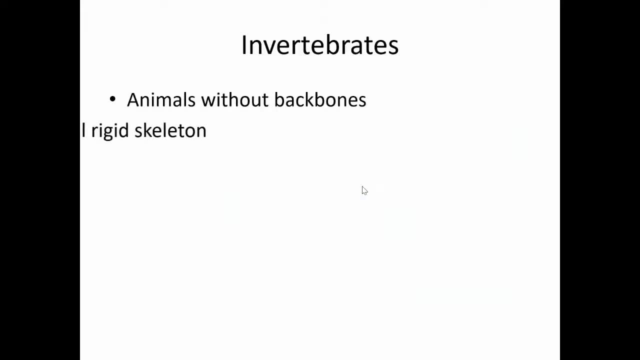 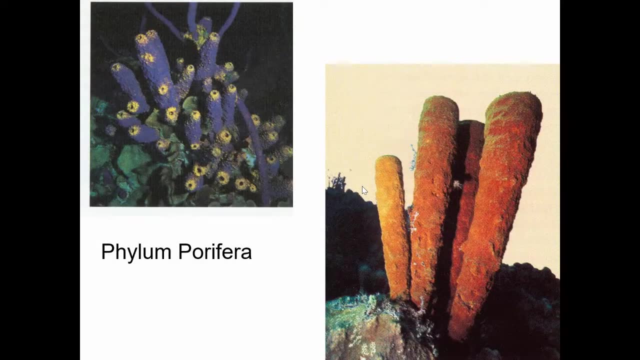 the simplest to those which are the most advanced. So there's a lot of text here. when you go through this PowerPoint on your own, I'm just going to highlight the picture portion so that we can get sort of the wow factor, but certainly feel free to go back and take a look at all the text slides as well. 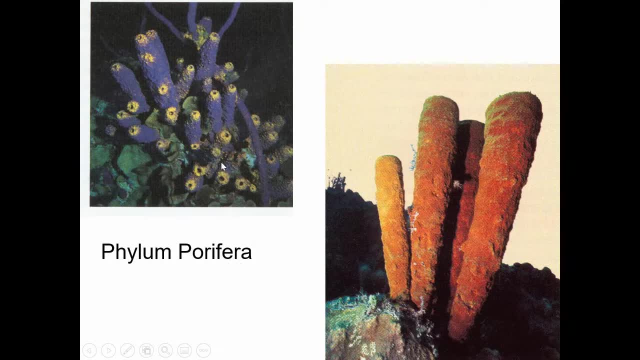 So sponges come first. Periphera means poor bear. It means it has holes in it. You can see them. There are large holes called ostia, and then smaller holes that allow it to filter feed. Sponges, of course, are benthic and they're found in all areas of the water column, and these are actually colonial. 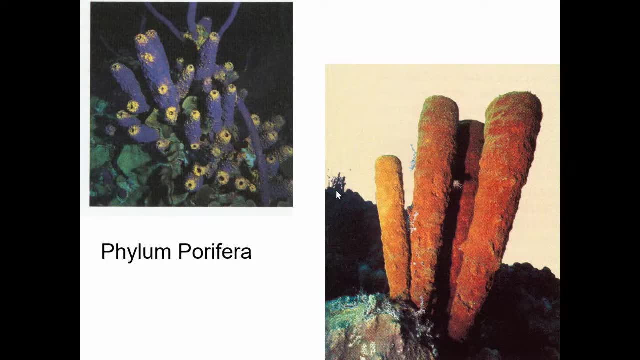 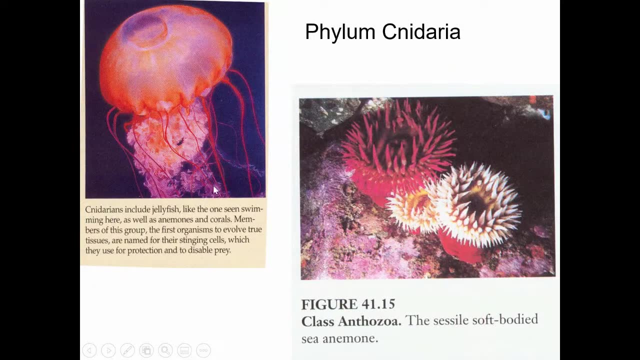 There are a bunch of cells living together with specializations, functioning as one simple animal. Next would be where our jellyfish come in. There can be all different types of jellyfish: Lion mane, local jellyfish like moon, jelly sea nettles and Portuguese man o' war, which we find in more. 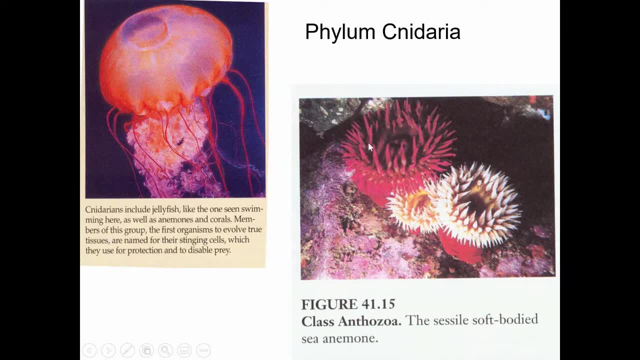 tropical areas. But if you flip the jellyfish upside down and glued its head, you'd get a sea anemone. These two are related, They both have the capability to sting and they're both considered cnidarians. But what's cool is: here's a. 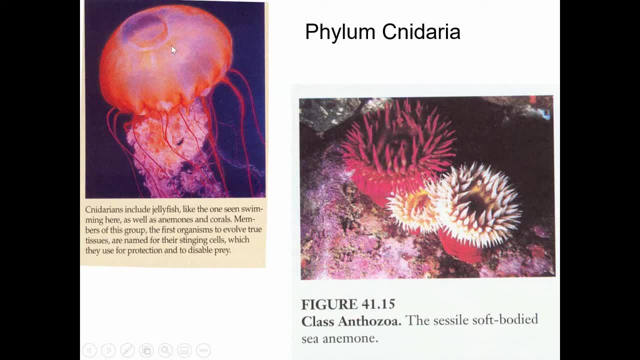 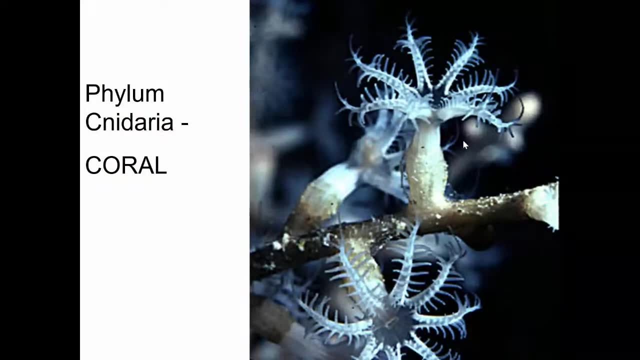 benthic example. Here's a planktonic example, right? So here's your pelagic and here's your benthic- Pretty cool Corals, by the way, as I had mentioned, fall in that same category, So these are what the coral polyps look like. 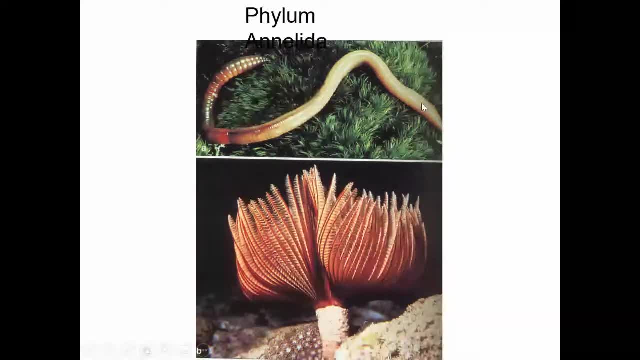 Worms fall in this category as well, and there are marine worms. So here's what an earthworm looks like. This is what we know. Here's what a fan worm looks like. This is the marine version. So we even have worms in the ocean. 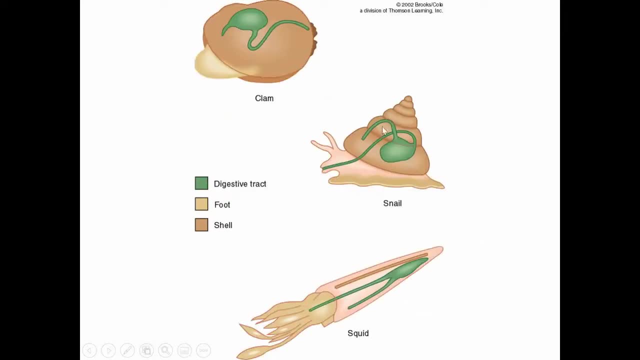 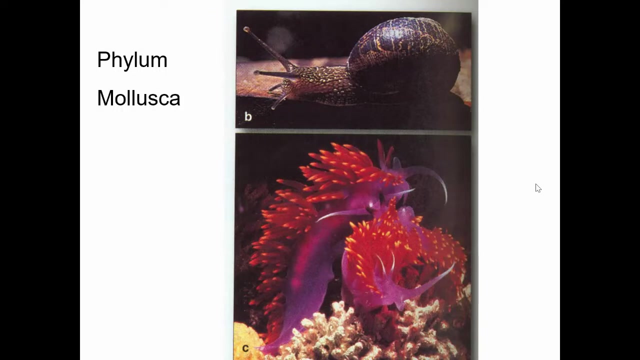 When we think about mollusks, anything that has a shell with a soft body, either inside or that can be exposed, whether it be a two-shell portion that can close shut one shell or a shell internal, that's what all of these represent, And so we have examples like snails. Again, we have snails on land, but we have naked snails or nudibranchs, as well as regular snails. Everyone knows what a conch is, right, Those are cool marine snails. We have some examples of scallops and mussels and oysters and clams. 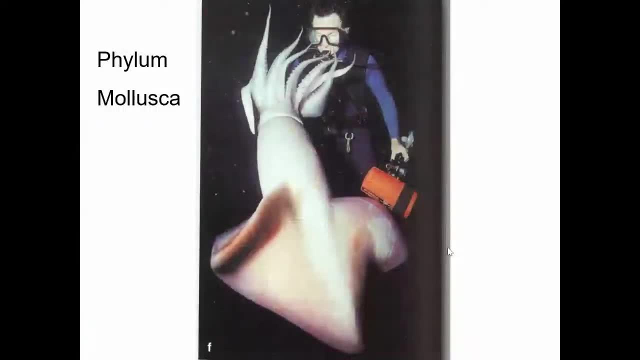 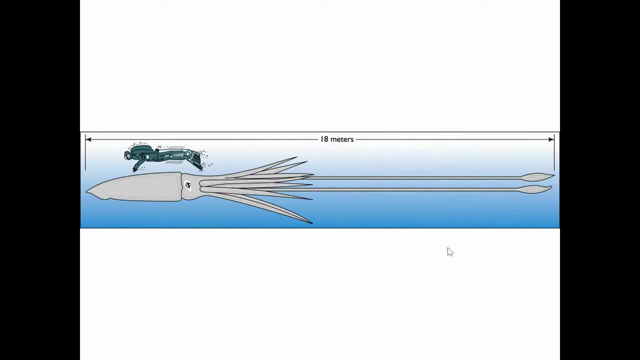 And we have a lot, some examples of cuttlefish, squid, octopus, all of these really cool mollusks. These organisms are tremendous in size And, as I had mentioned, they're even tied into the largest animals on the planet, the whales. 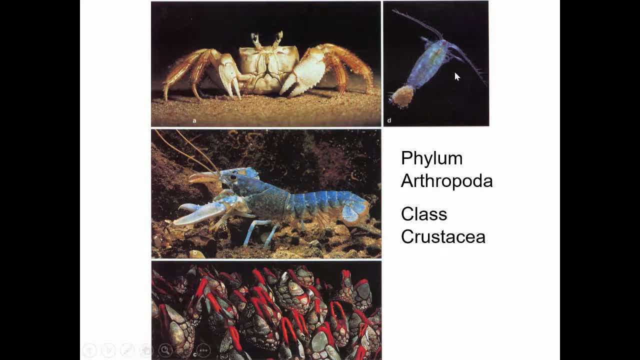 The arthropods or the jointed appendage organisms are the ones that come next. You've already seen this guy here. This is a copepod. This fits into our zooplankton category, But in the adult stage we can have crabs, lobsters, shrimp, amphipod, isopod. barnacles are represented here. 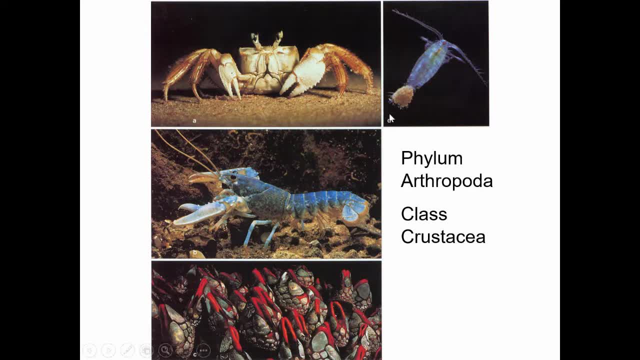 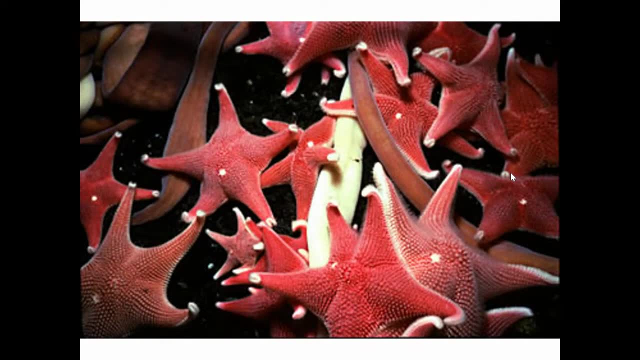 These guys all are benthic in their adult stages or remain planktonic, depending on which one we're talking about. Finally, from an invertebrate perspective, the econoderms represented here by a sea star or five-pointed radial symmetry. There's a central point that sort of radiates from the middle, almost like your hand right. 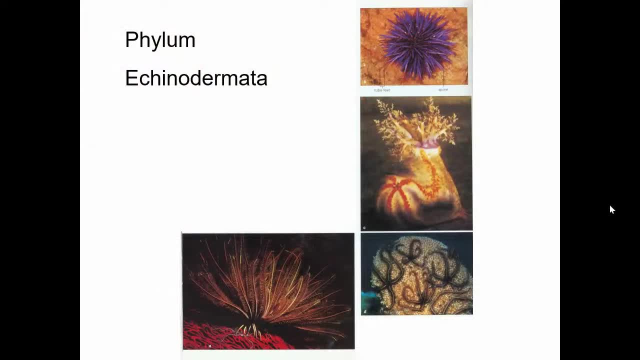 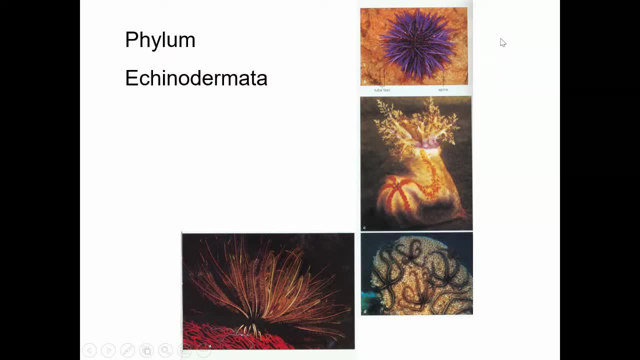 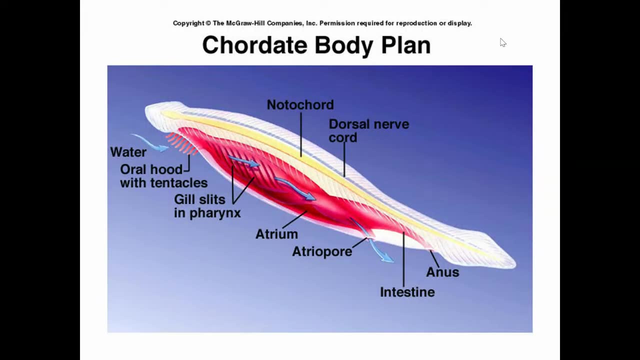 And then, of course, the conch, That would be a brittle star, sea cucumber, sea urchin- Many of you have seen those. We call those the pin cushions of the sea Moving on from our invertebrates. animals without backbones would be vertebrates. Vertebrates would be us. right, We have a vertebrae, a spinal cord. 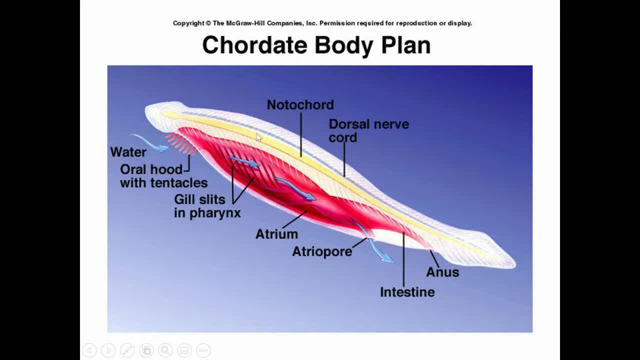 So now you see where the word chordate comes from. Chord means cord. The cord originally starts along the dorsal part or the back part of the body, as being a notochord, which means not cord that has a nerve bundle in it. 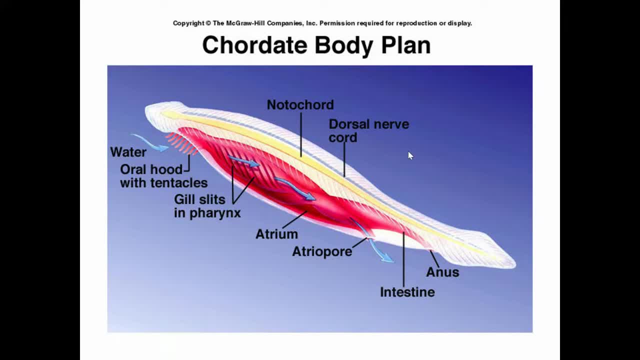 If you think of your spinal column right, it's a bone that has nerves that run through the center. Well, so our original body plan functioned the same way. We ate from one side, We excrete from the other side. We have all of our organs in between. 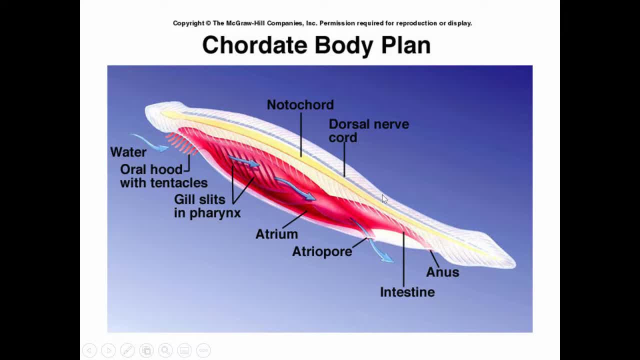 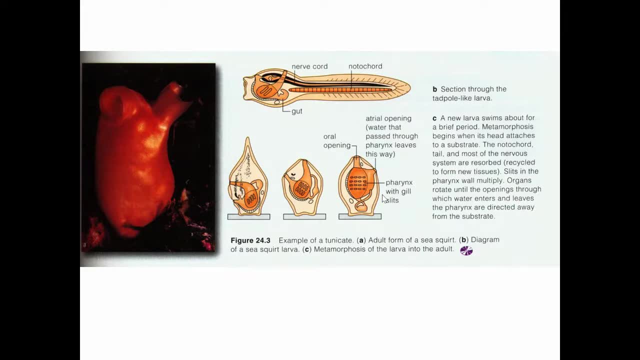 And we have a cord that helps us stay upright. Well, fish have that cord running along their backside, And so we actually have to have an evolutionary link between the invertebrates and the vertebrates, And they are represented by tunicates, sea squirts, amphioxus lanceolets. 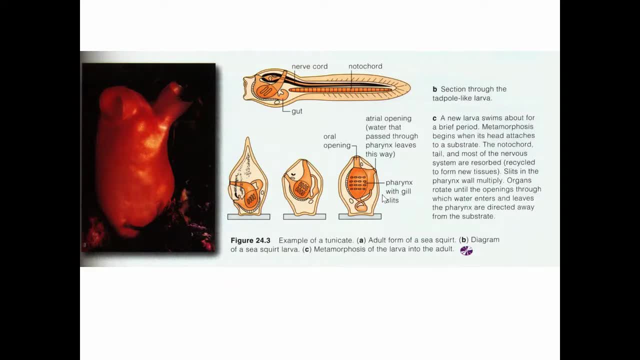 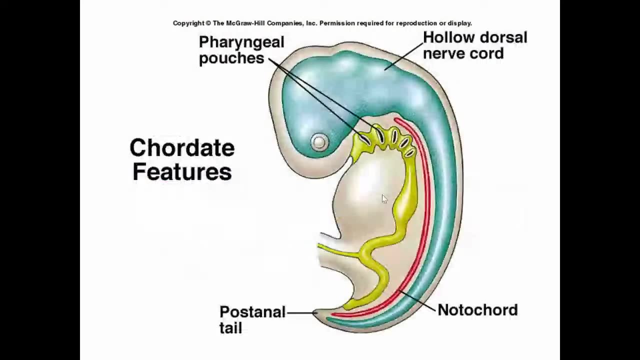 And all these vertebrates And all these other cool organisms, simply because they have this internal notochord or notchord. They don't look like much but believe me, from an evolutionary perspective they are extremely important. When you get to the true chordate features, you still have that notochord or notchord with the nerve bundle inside. 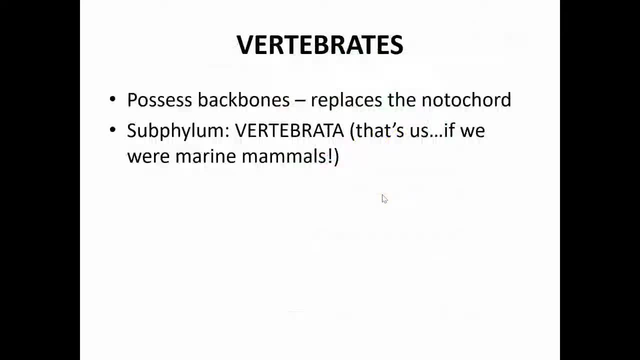 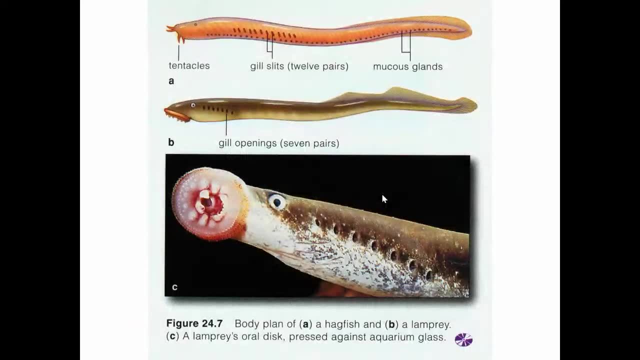 But you also start to develop some other unique capabilities. That cord will eventually harden to become a vertebrae. That vertebrae will eventually become bone, The organisms that you know here. They represent the mammals, right, But before we can get to mammals, we have to get there from an evolutionary perspective. 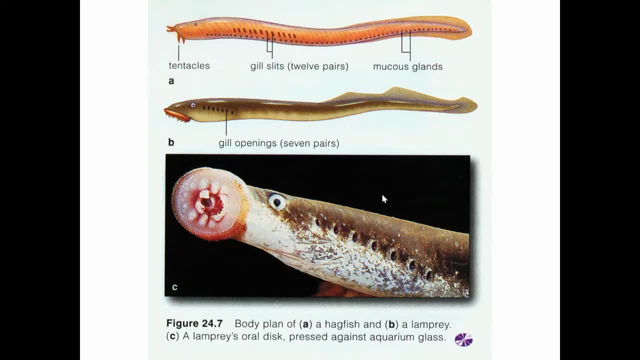 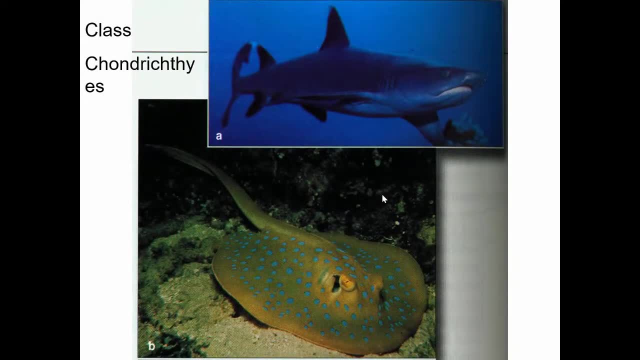 So we have three categories of fish, represented by the hagfish and the lamprey. They have these really cool mouths. The next category of fish: we have stingrays and skates, as well as sharks. You're starting to see more familiar faces now. 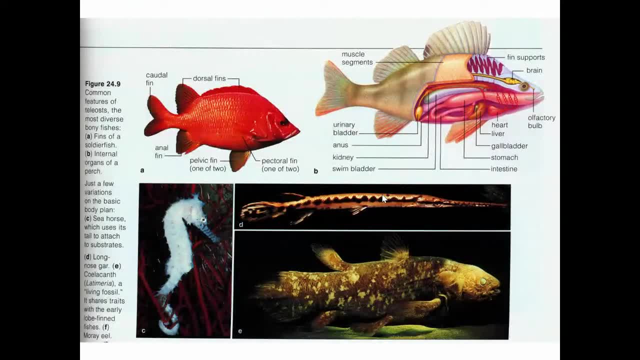 As well as the true classic fish, right. And fish can come in all different sizes and shapes. Seahorse, Seahorse- that's a fish, right? It's not some crazy alien organism. These are all bony organisms, right. 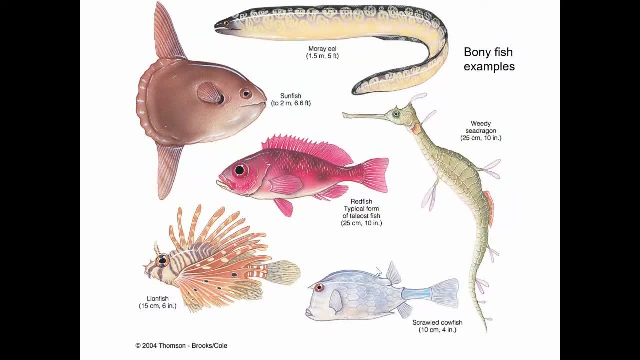 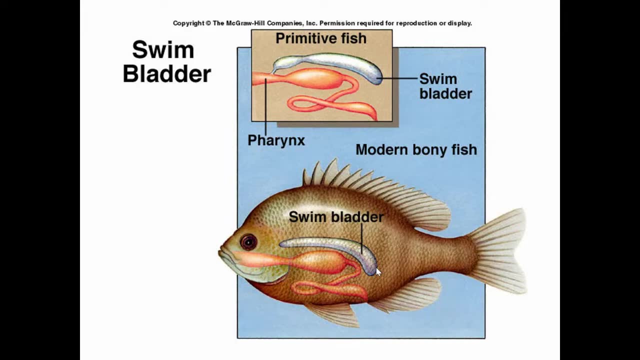 Bony fish, bony chordates. Once we leave the fish category we get to the reptiles, the birds and the mammals. In order to have those changes from fish to reptiles, birds and mammals you have to have some differing capabilities internal. 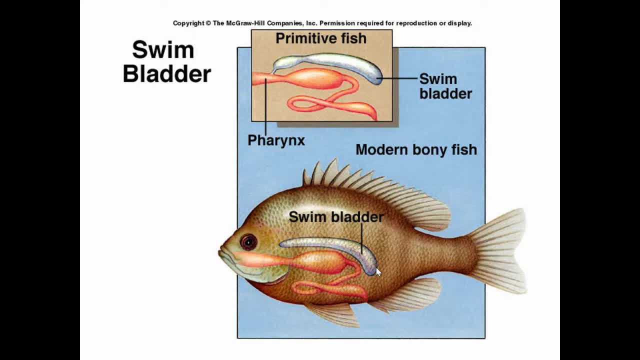 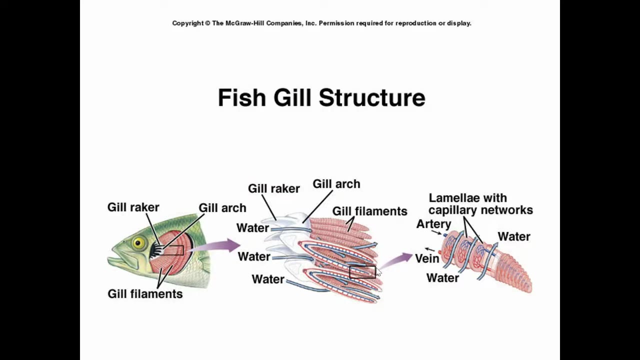 Remember I talked about fish living in the water column versus in the deep. We have some capabilities of these balloons or swim bladders that can inflate or deflate To allow for buoyancy and to allow them to remain in the water column. If you're a reptile, a bird or a mammal, you're going to need to have that capability or lose that capability. 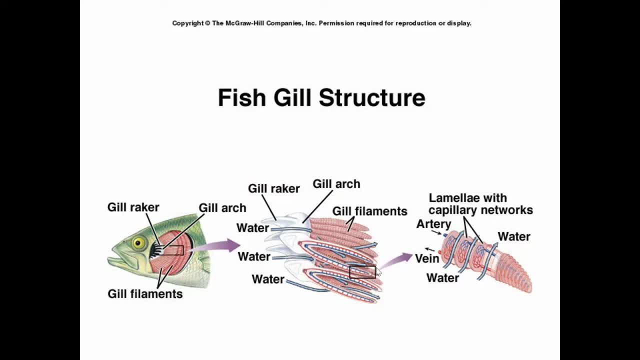 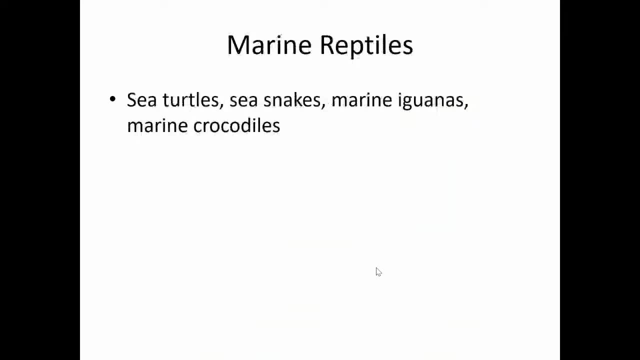 But also now start to have the ability to have life on land. So we're going to start to change the gill structure and the capability of oxygen exchange in a fish to a reptile right. We don't have gills exposed here anymore. 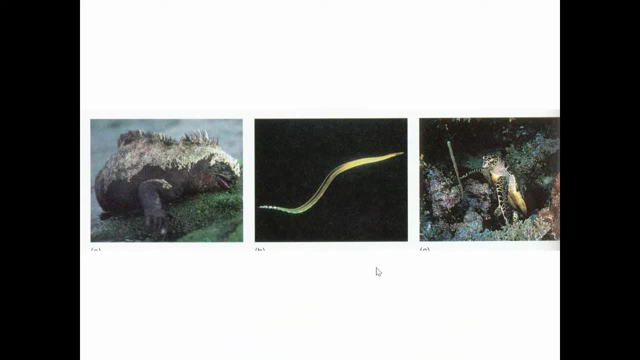 Classic reptiles are iguanas, sea snakes, turtles. We also have crocodiles that fall in this category as well. These guys are also chordates, but they have a thick leathery skin and they have the ability to breathe on land. 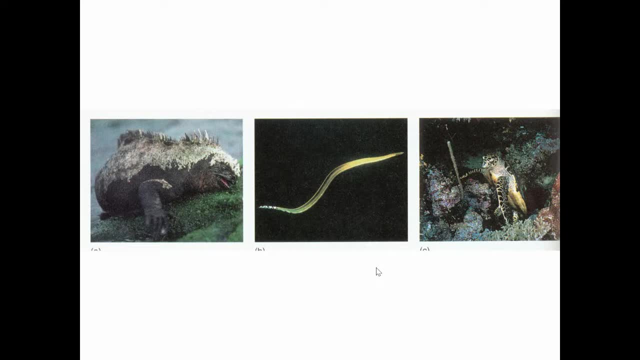 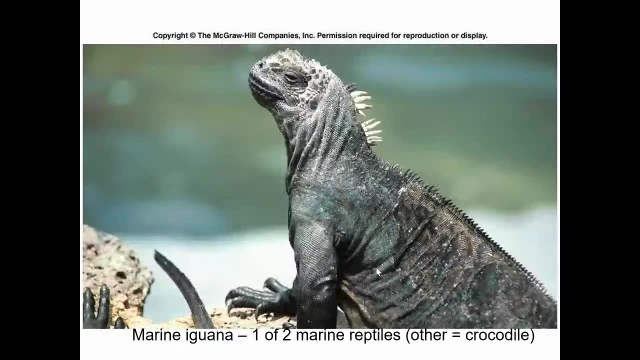 Not all of them. Some of them have modified lungs and different capabilities, but most of them have the ability to crawl out on land And some of them even need to crawl out on land to rest, nest feed and breed. They're also cold blooded, which is kind of cool. 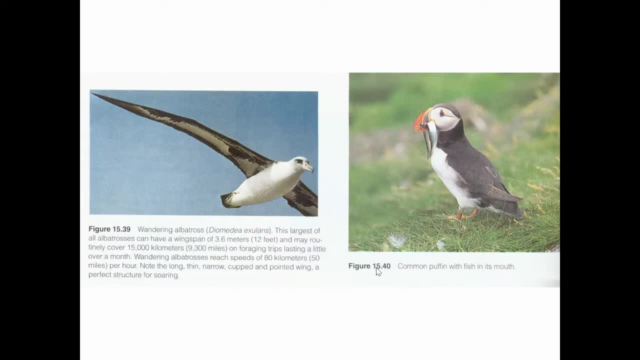 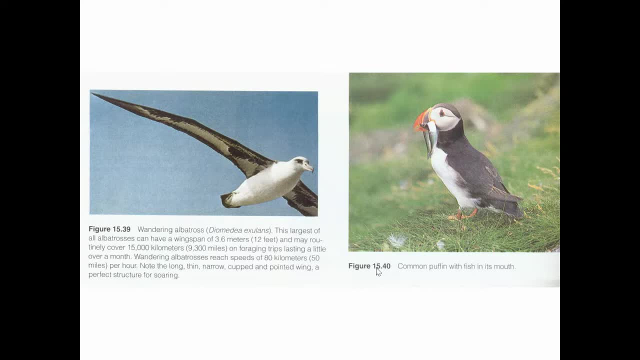 that are integral components to the marine trophic structure: Puffins, penguins- those are the classics. You've all seen seagulls flying about the shoreline, but there are albatross and other amazing birds that can fly hundreds of miles and that live on rocks in the middle of the ocean. that 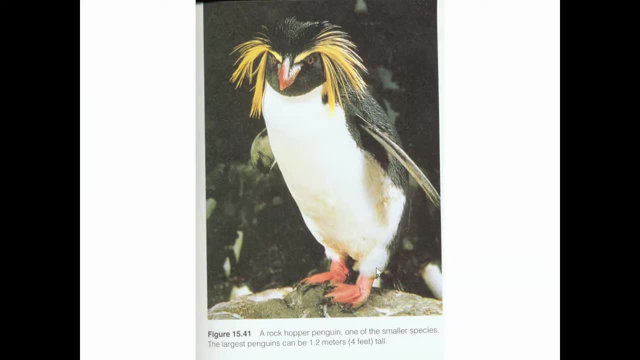 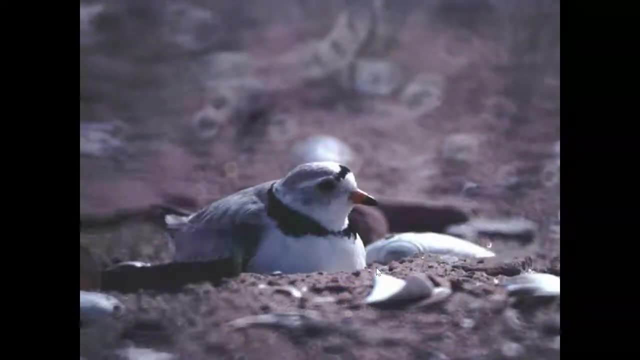 have the ability to feed Penguins, of course, live along the shoreline and then they walk along the ice sheets to be able to hatch their young. One of our local most famous birds everyone that we love to hate is the piping plover. These guys are the ones that nest on our beaches and get our 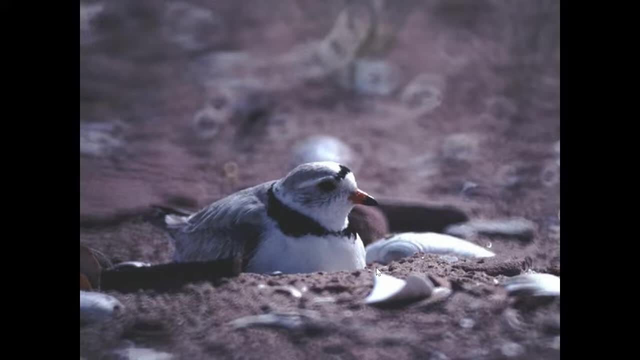 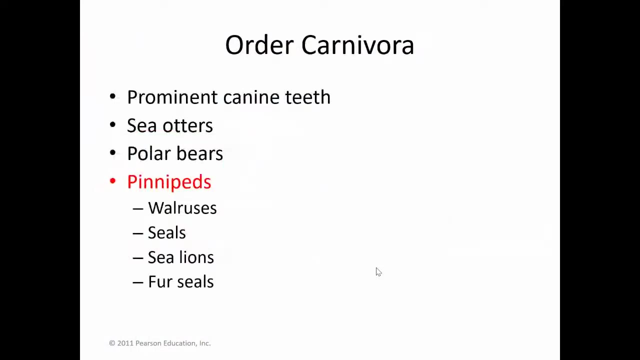 fireworks canceled and stop our ability to drive our cars or even build houses on the beach, because they're a protected and threatened species. Finally, at the very end of our evolution, we get to the mammals. The mammals are what we know. These are our charismatic megafauna. They end with: 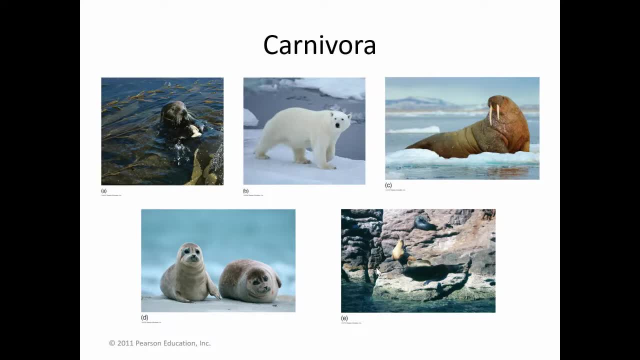 the whales. right Before we can get to the whales, remember, think of the evolution we just had. We went from invertebrates without vertebrae to vertebrates, those that have a spinal cord that hardens right, A true vertebrae. From there we had the fish, reptiles and birds. We ended up. 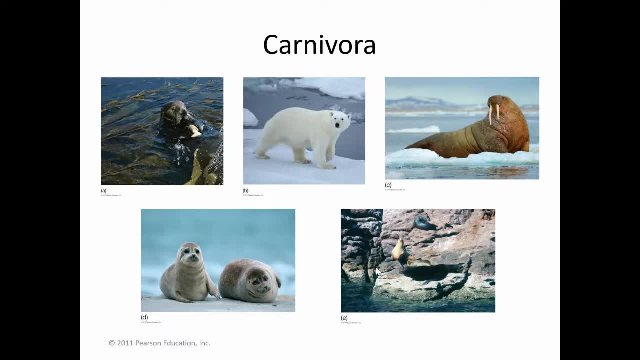 getting warm-blooded. and now we end up with the different types of mammals. Mammals fall into a bunch of categories: carnivores, pinnipeds, sirenia and cetaceans. Okay, so we're going to in the carnivore category. Carnivore, think meat eater. right, We have classic examples like a sea. 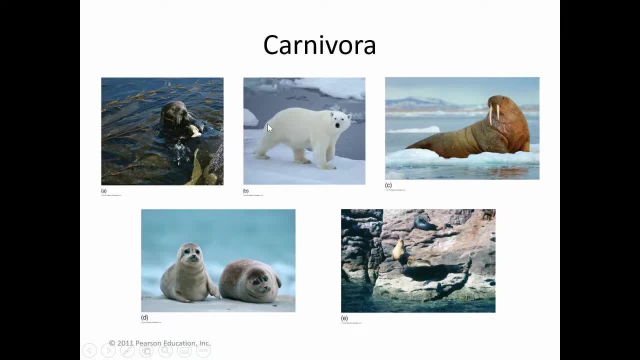 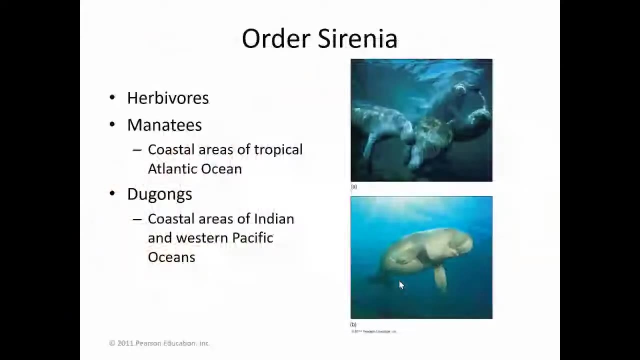 otter and a polar bear, whose bodies are completely covered by fur or other. probably also equally popular and equally famous carnivores such as the walrus, the seal and the sea lion Elephant seals fall in that category as well. Pretty cool organisms. The sirenia are the. 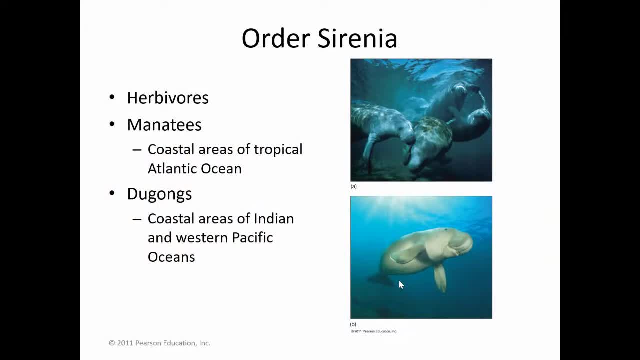 manatees and dugongs. Those of you that have spent any time in Florida, these might become children for you. These are another classic example of a really large organism. depending upon a first-level trophic structure, These guys feed exclusively on grass. They are vegetarian, That's. 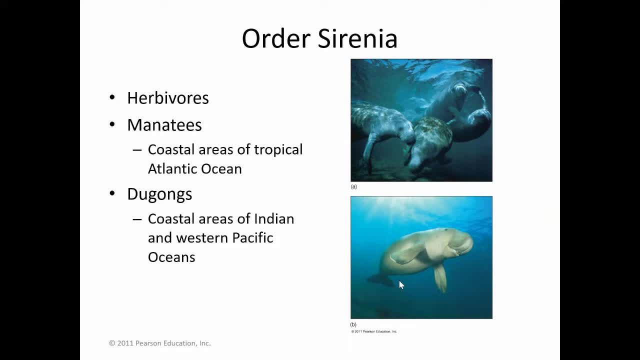 why we hear them called sea cows. So if we get rid of the primary producers in the ocean by polluting our water, by not having the ability to have plants, these guys lose their food source and then we lose the manatees. So you'll often see save the manatee stickers all over Florida for 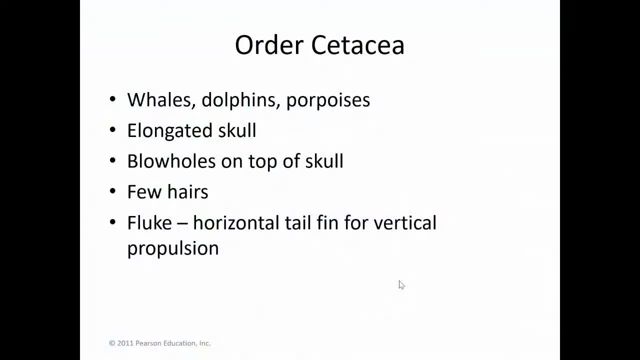 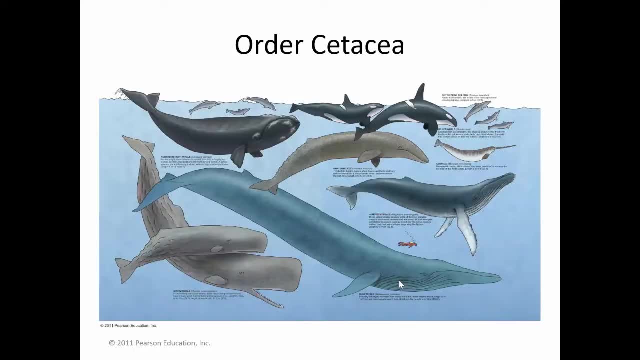 that reason There's a mother and calf Beautiful picture. And finally, when we get to the end of the line, the cetaceans. this is where our whales fall in And this is essentially how we started. Our whales come in two versions: the baleen whales. 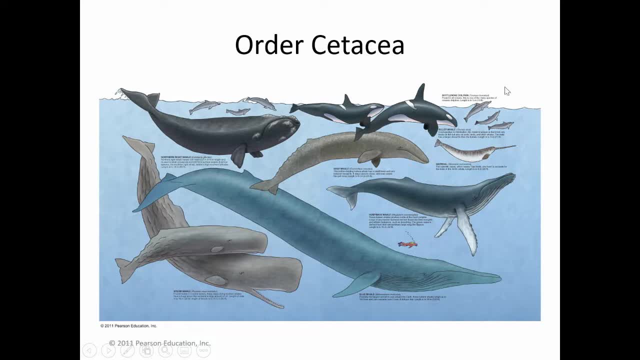 those which filter feed and the toothed whales those which don't. And it reminds you that we have this giant link from the smallest things in the ocean to the largest things in the ocean, and that each and every one of those is worth saving, worth protecting and worth understanding. And so what?